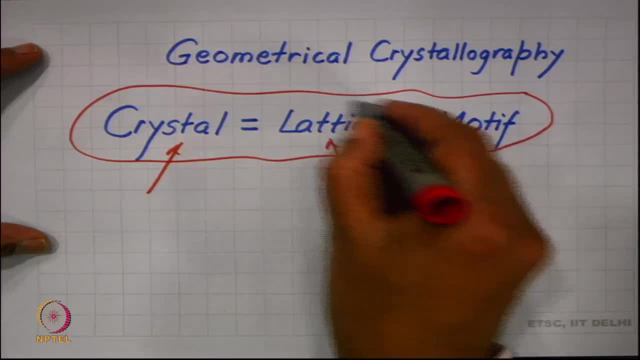 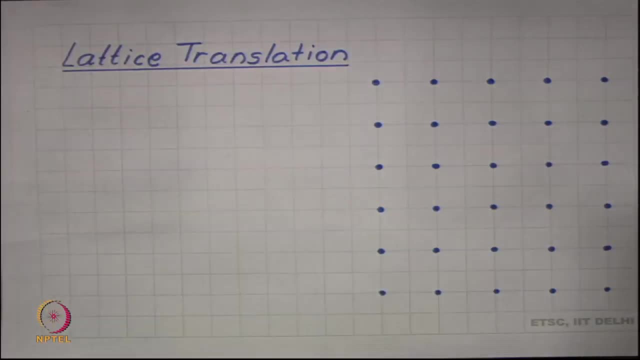 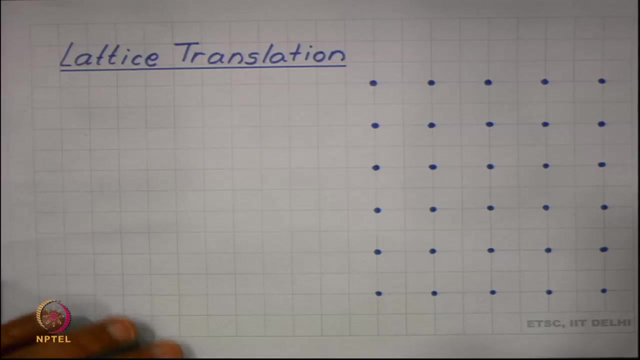 bit more detail about some of the properties of lattice. So lattice will be the focus of this session. We begin with lattice translation. We already have a periodic set of points which is a lattice, and I have drawn an example here: a nice simple square lattice, Lattice. 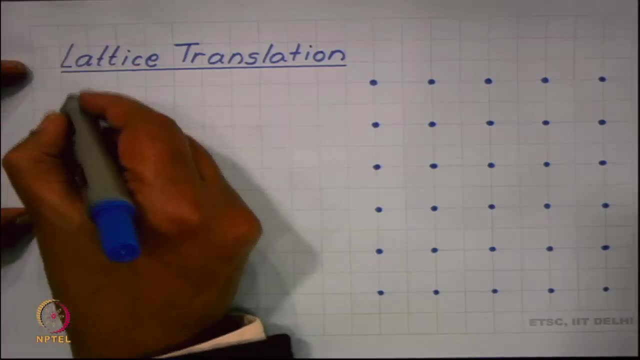 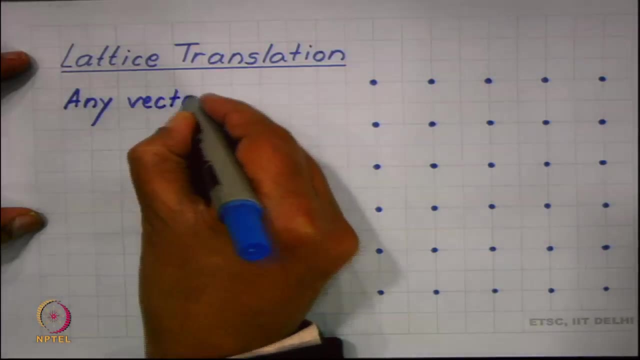 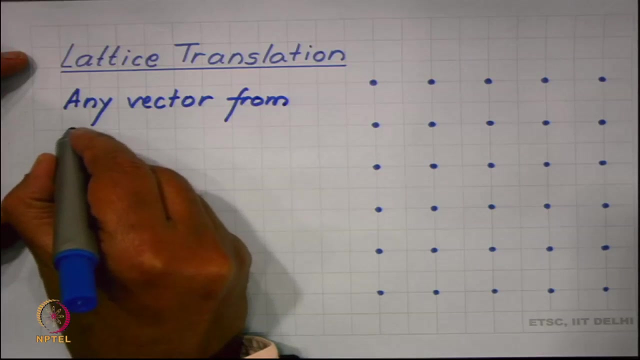 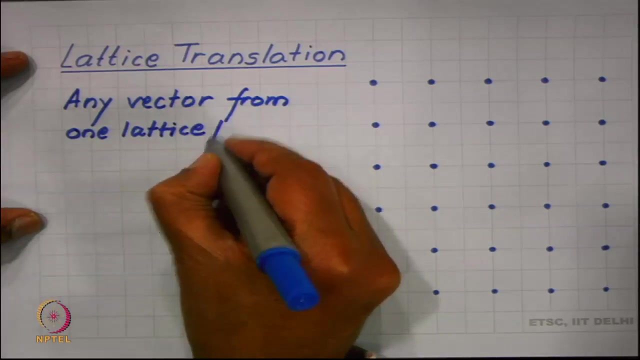 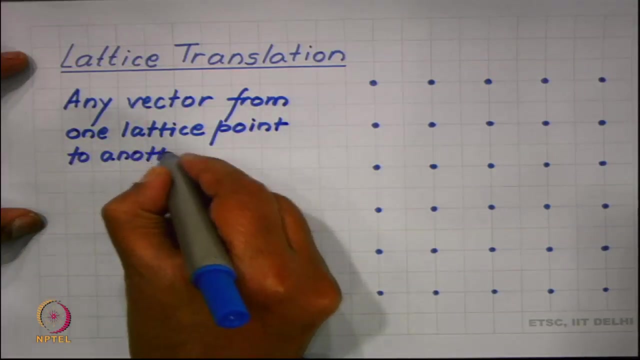 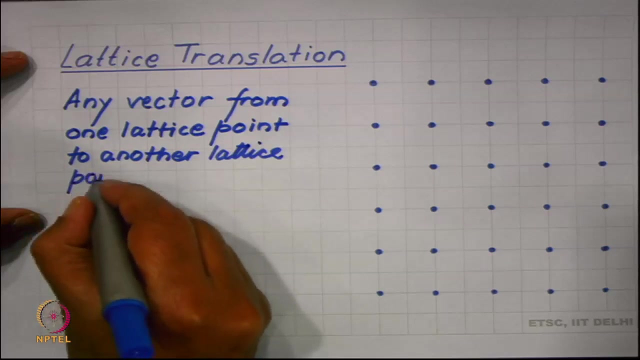 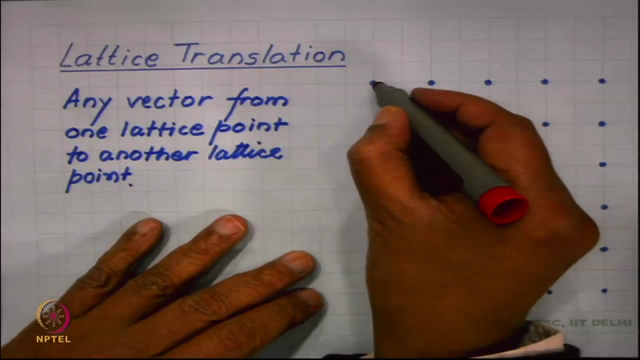 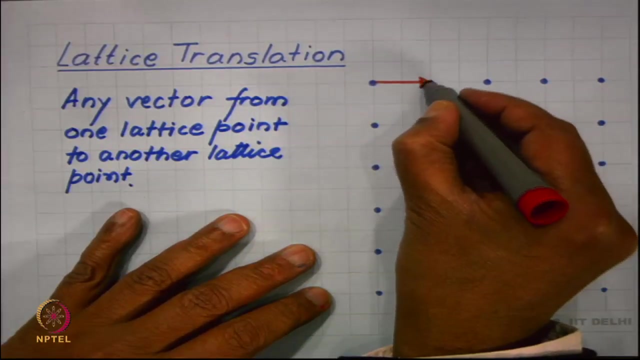 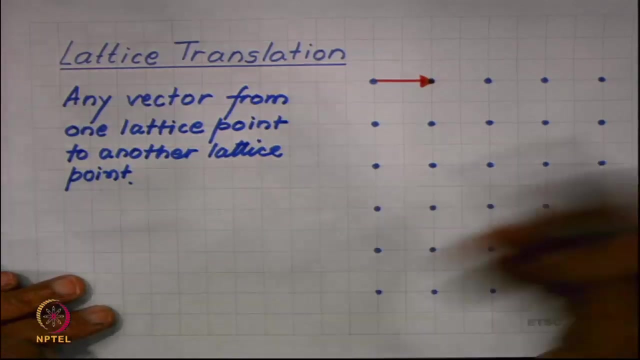 translation is: we can define as any vector from one lattice point to another lattice point. I will draw some examples here. So, for example, I take this, this as my lattice point and I draw a vector, horizontal vector. Okay, I can draw a vector up to the next nearest neighbor in the horizontal direction. So 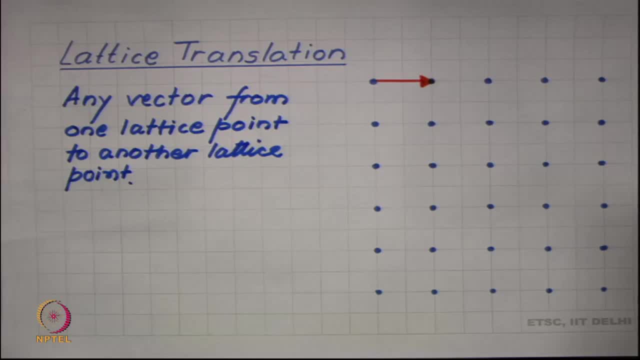 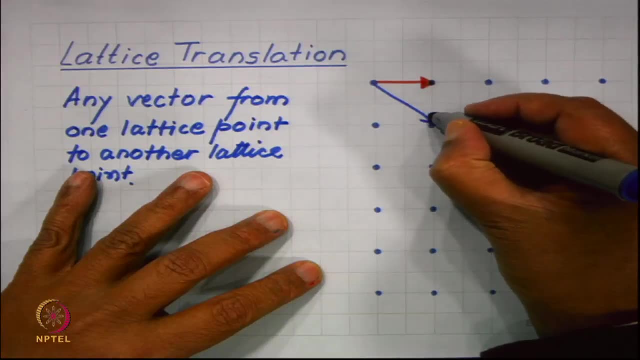 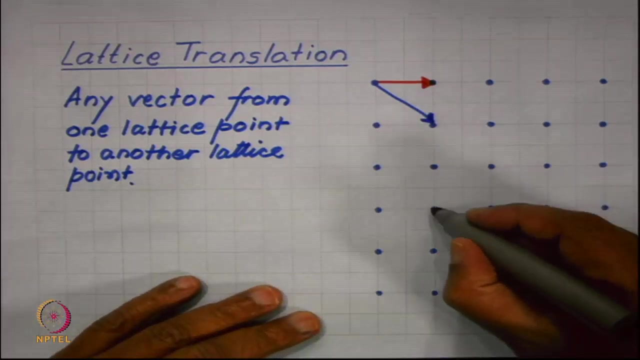 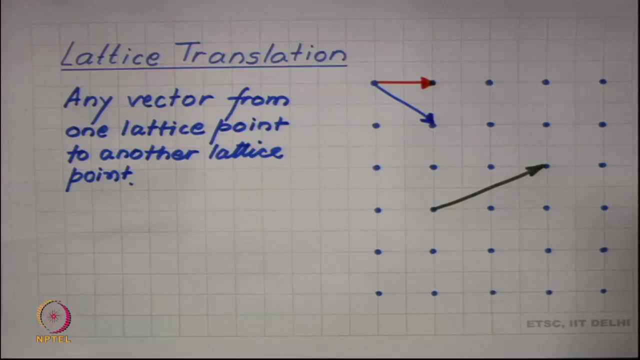 this red vector is an example of a lattice translation. Or, if I wish, I can draw another vector like this: This is also a lattice translation. or yet another. I can start from here and draw this vector: Okay translation. So all these vectors are lattice translation. Of course, a lattice will have. 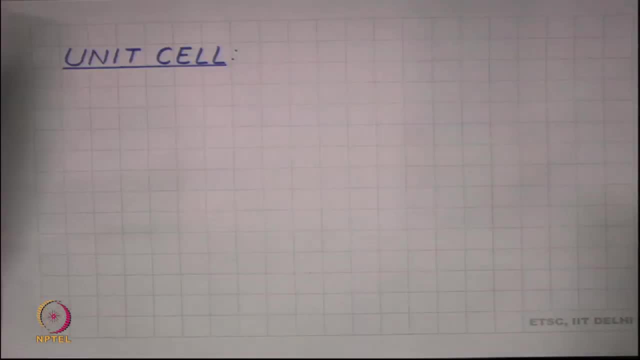 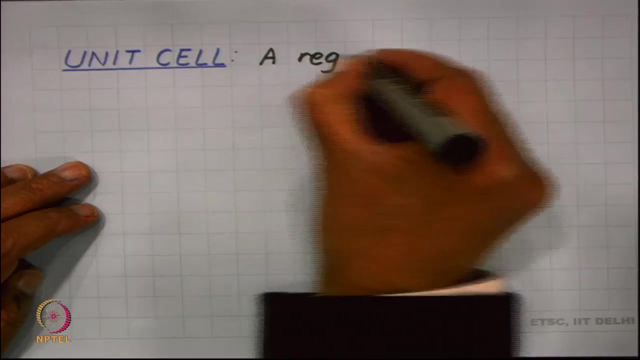 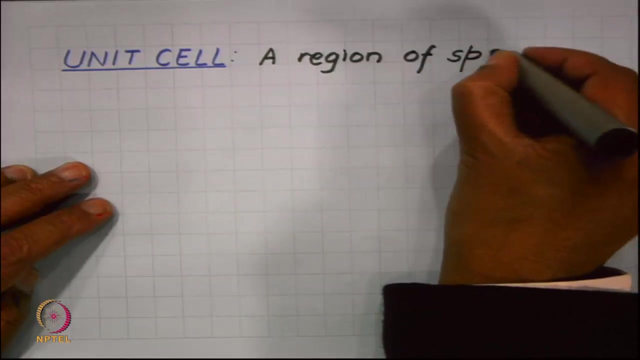 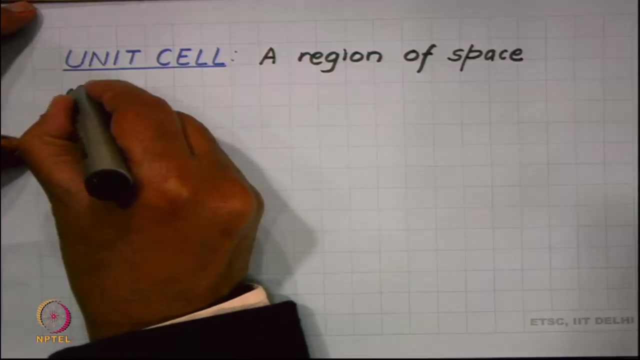 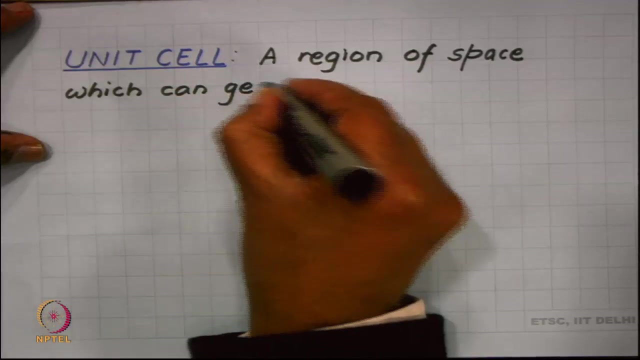 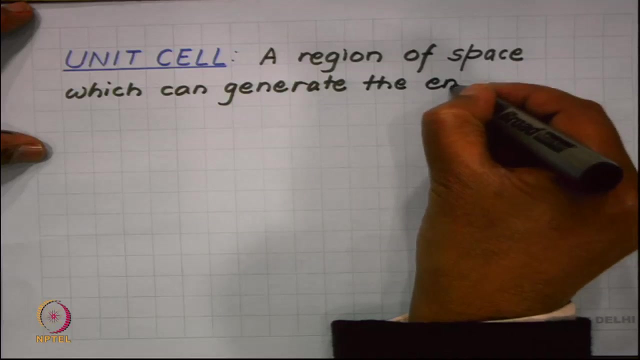 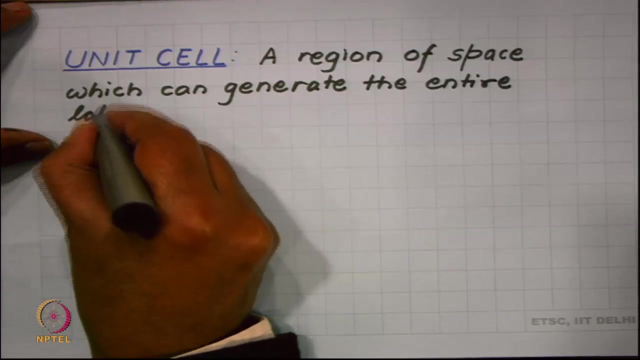 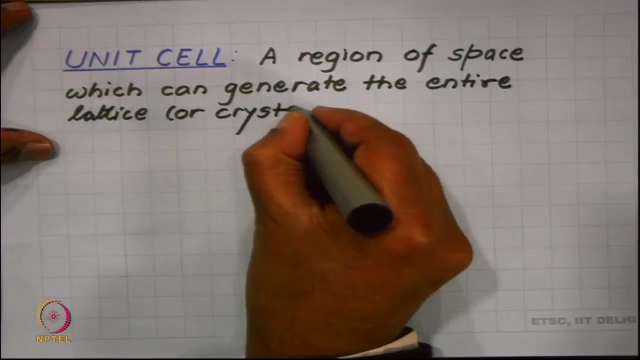 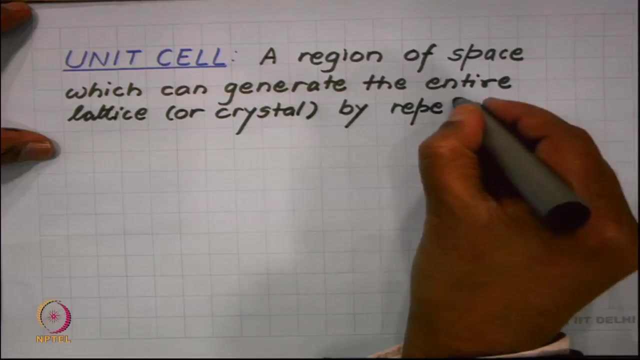 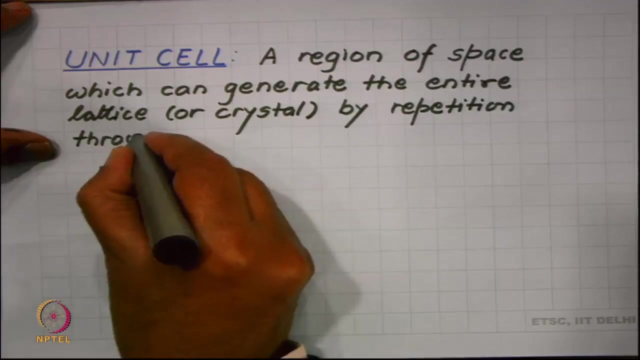 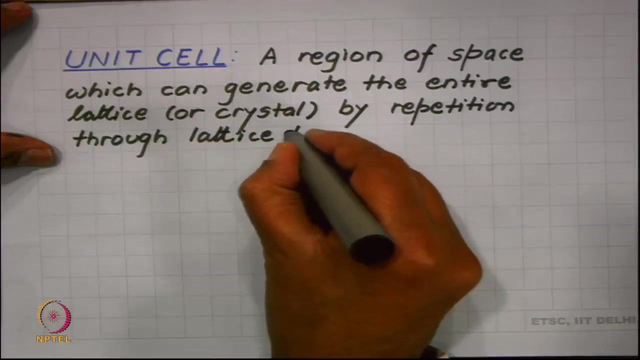 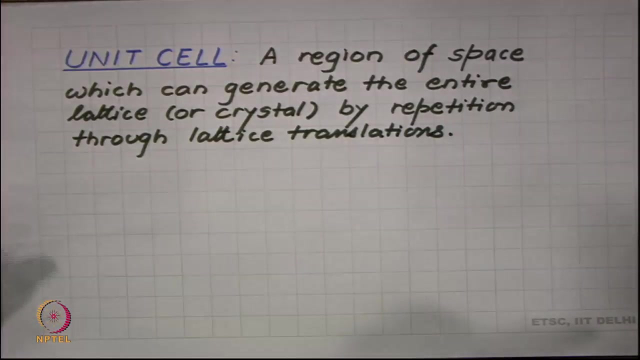 many such lattice translations. We will now define a unit cell. Let me first give a little abstract definition. So I will define a unit cell as a region of space which can generate I the entire lattice or crystal by repetition through lattice translation, So connected. region of a space which can generate the entire lattice. 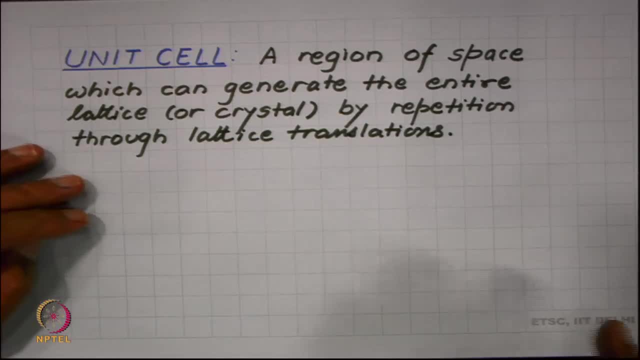 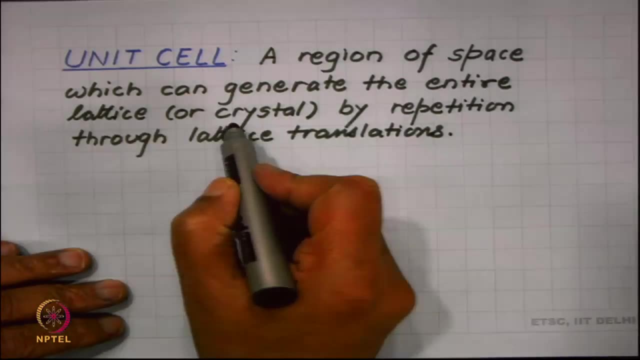 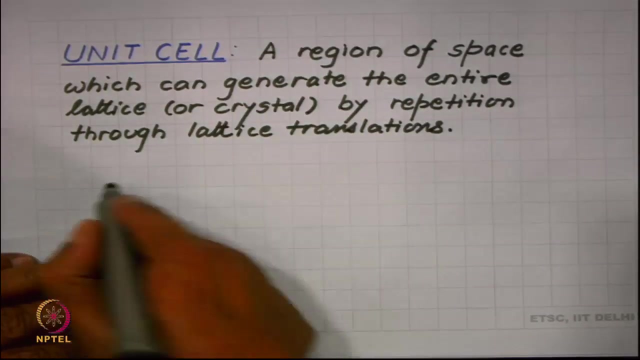 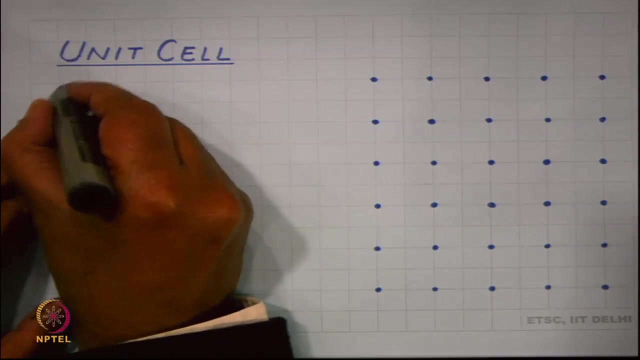 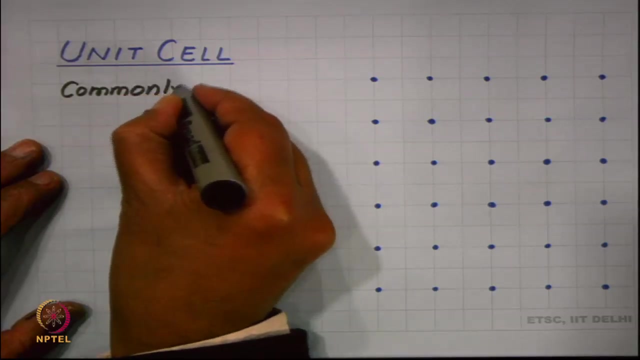 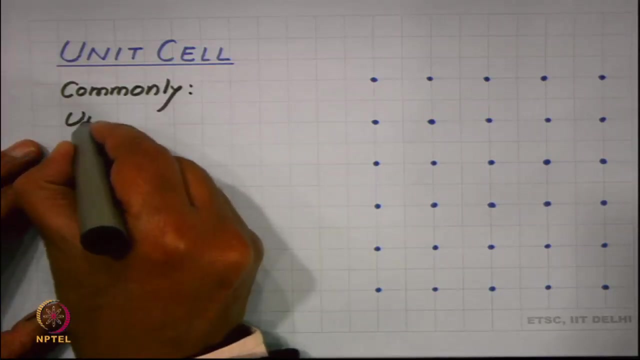 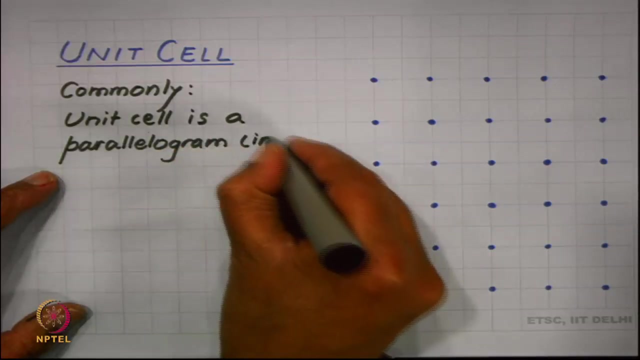 By repetition through lattice translation will be called the unit cell. The unit cell can be either of lattice or of crystal. We will see. let us see some examples. So we have commonly, although that is an abstract definition. Let us say a unit cell is selected. unit cell is a parallelogram. parallelogram in 2D. 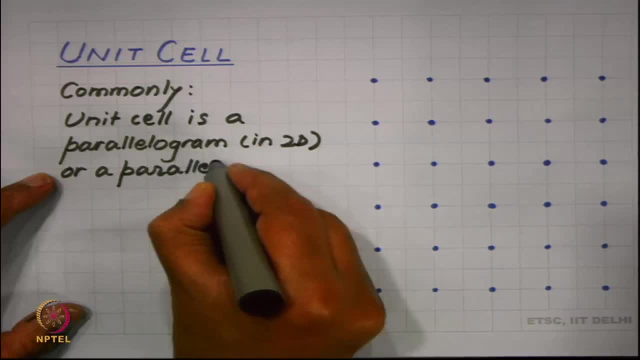 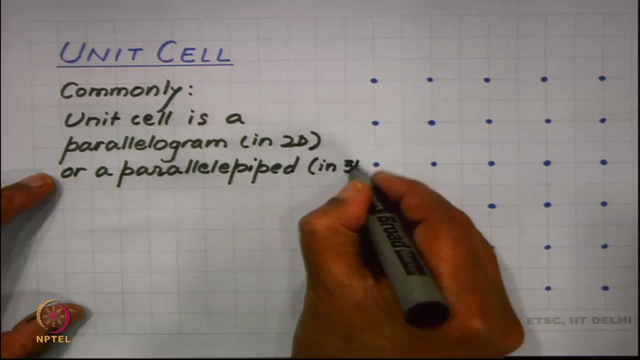 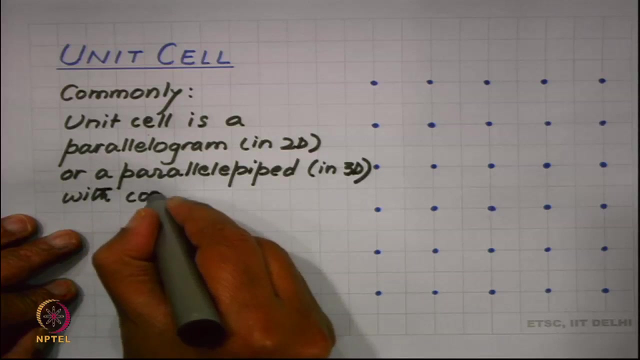 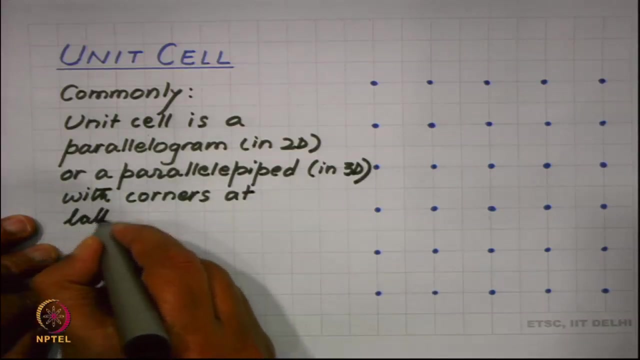 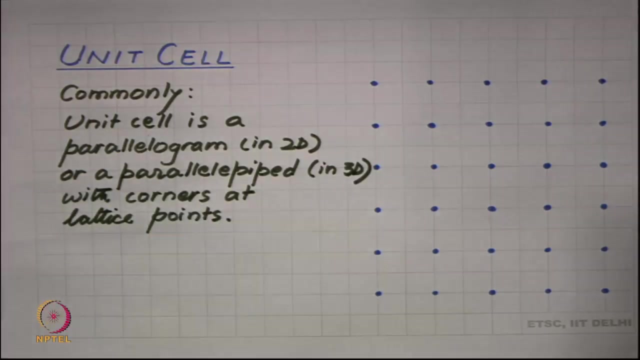 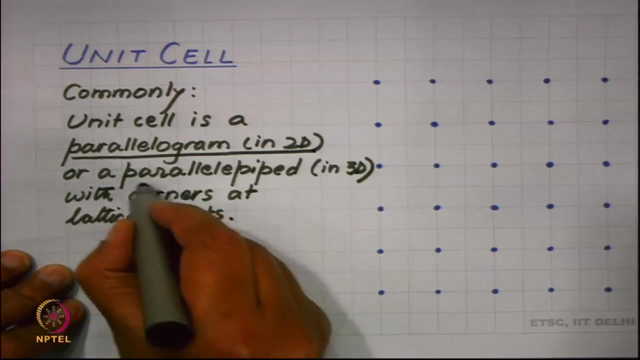 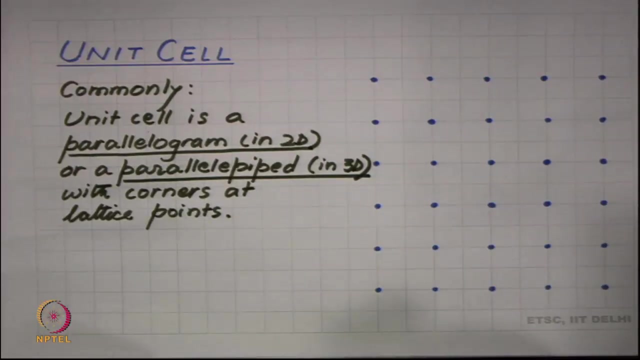 Or a parallel pipette in 3D, Or a parallel pipette in 3D with corners At all time lattice points. Different shapes can be selected, but the common shape which is selected is a parallelogram in 2D or a parallel pipette in 3D. So again I have an example of a 2D. 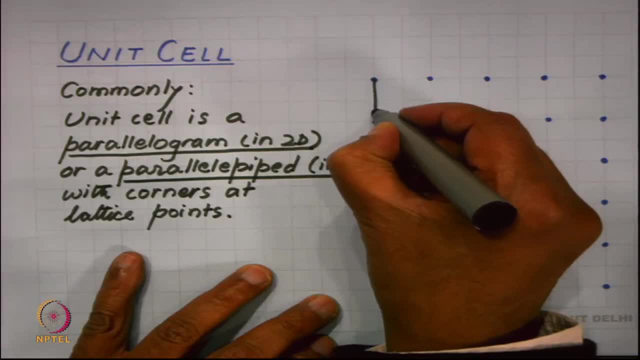 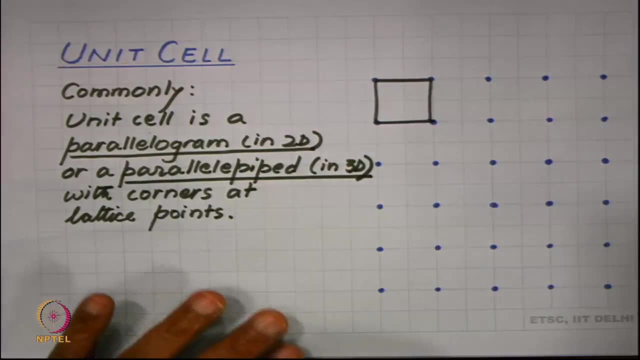 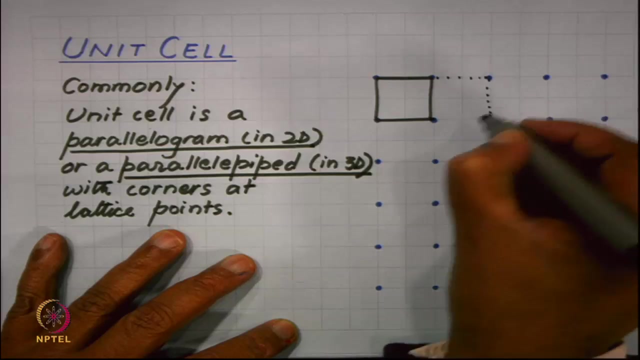 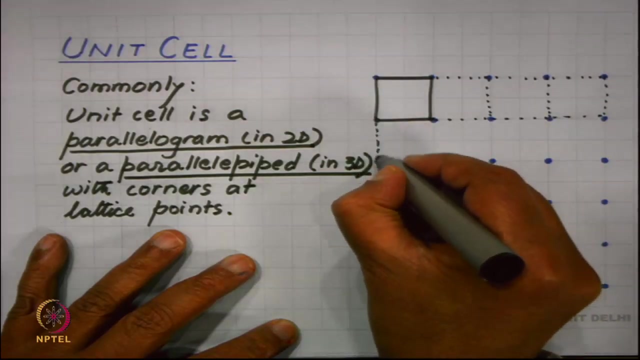 lattice here and if we wish, we can select a square in this lattice. this square will be the unit cell, Because if I repeat this square, this square has corners at the lattice point and if I start repeating this square, I see that I can get the entire lattice all. 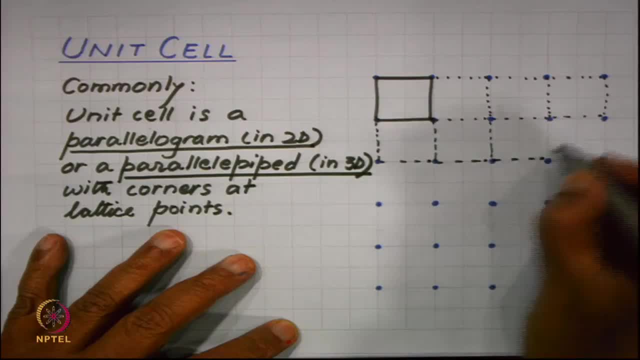 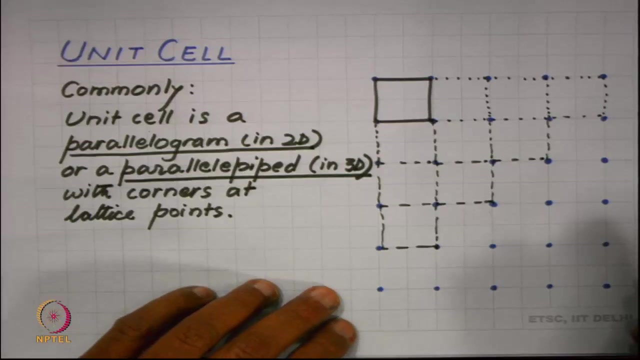 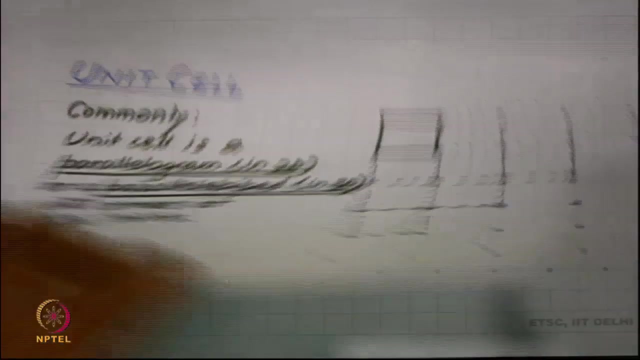 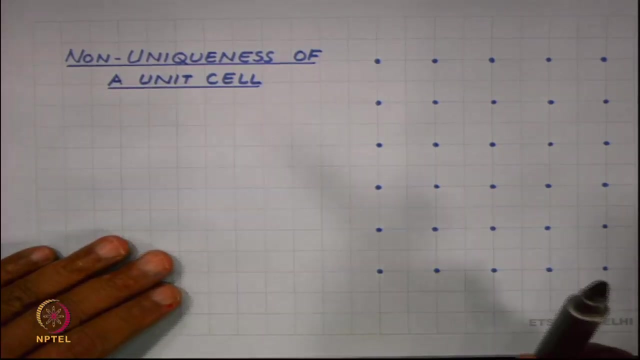 the points can be obtained by this Such a repetition. So I have to periodically translate these unit cells and I have to recognize that lattice points are at the corners. However, a given lattice has not one unit cell but many different lattice points. 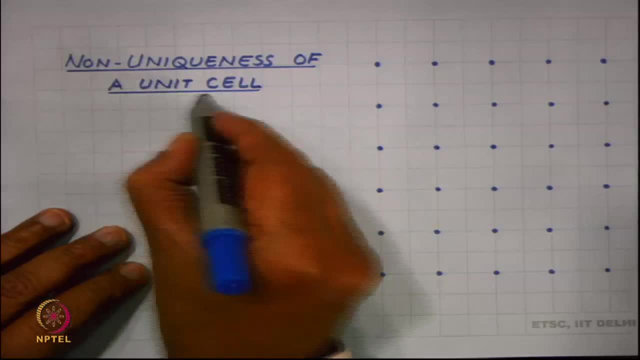 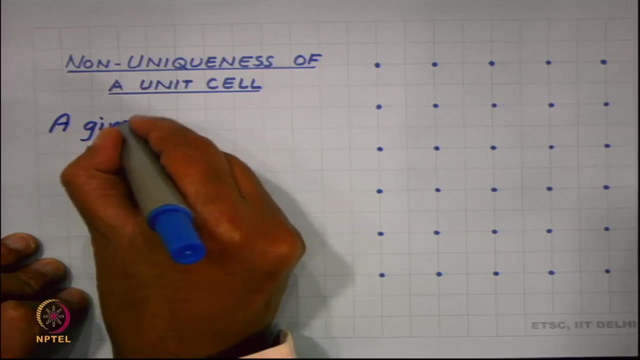 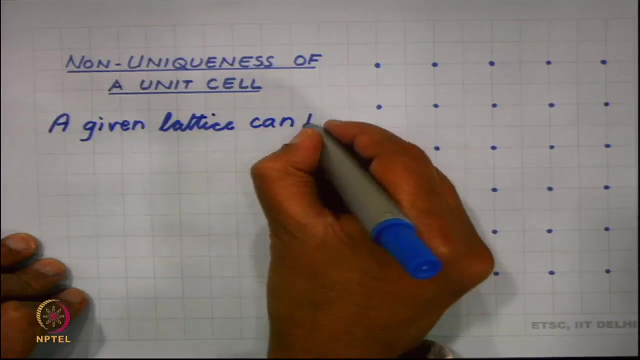 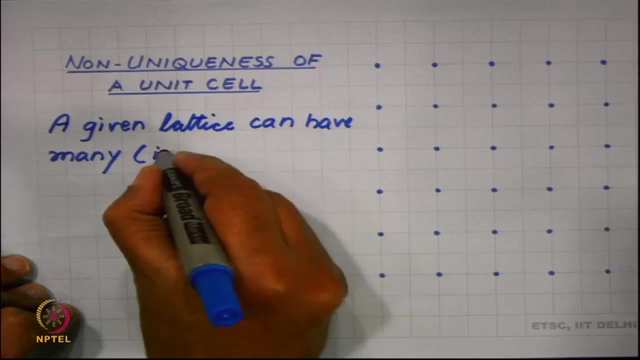 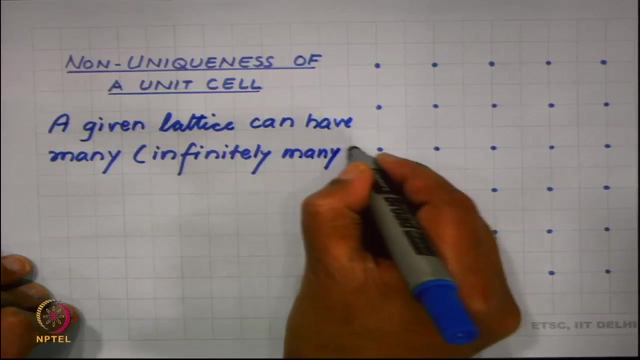 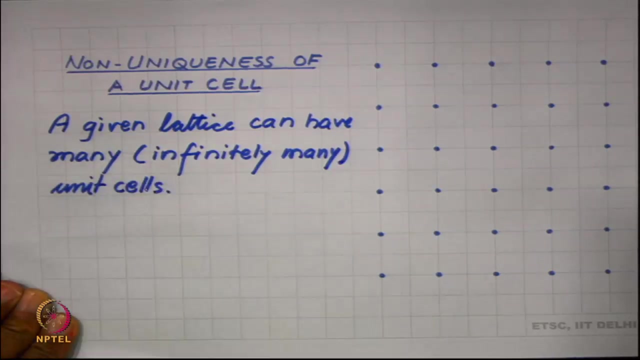 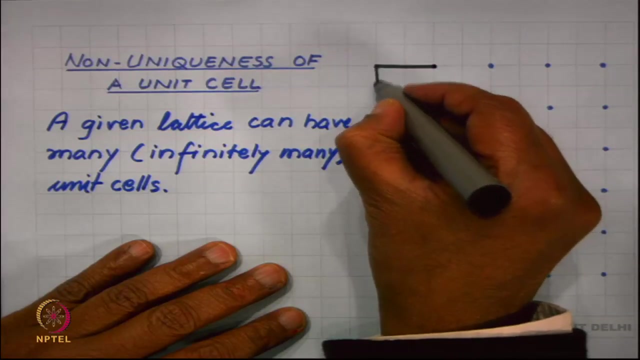 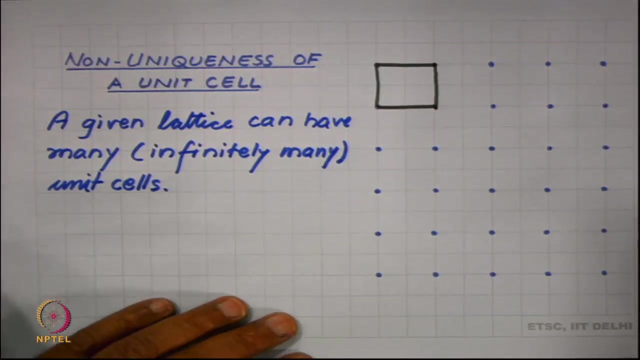 Different unit cells. So the unit cells are not unique. A given lattice can have many, in fact infinitely many Unit cells. We will see here, for example, in the same square lattice. initially we had selected a nice square as our unit cell, But in the same lattice. if I show this, I can. 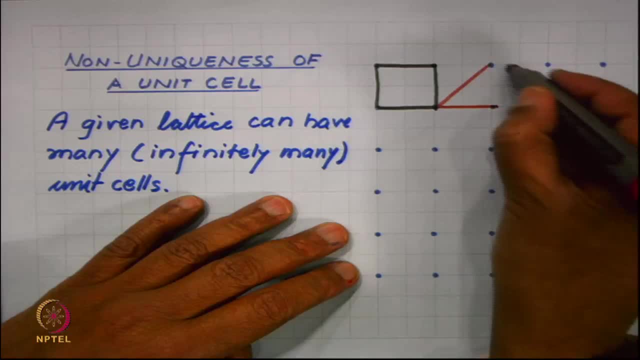 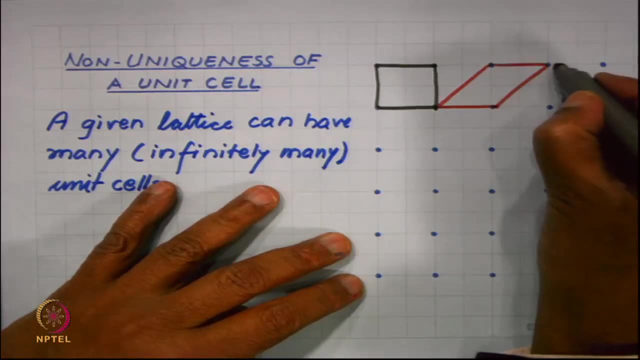 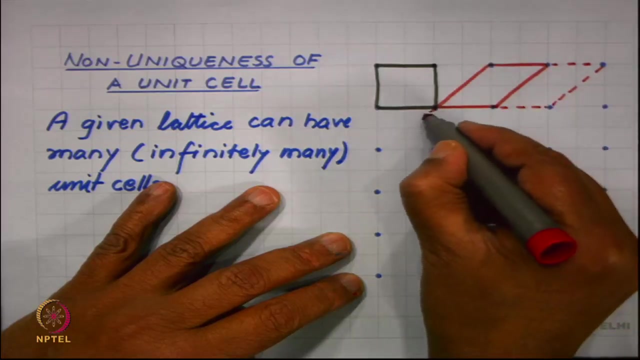 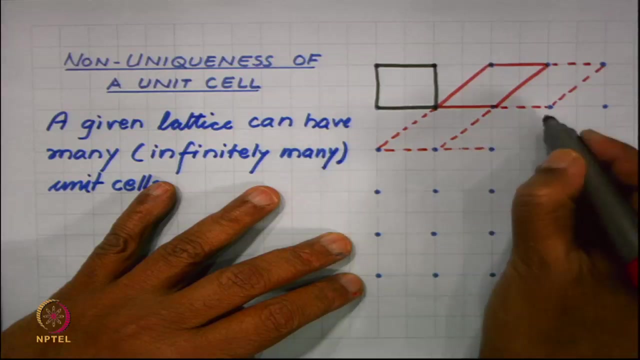 select Unit cell, This red unit cell, which is no more a square but a parallelogram, And if I repeat this parallelogram, I again can generate the entire lattice. So what happens here? So what I want to do is I take a block of lattice. 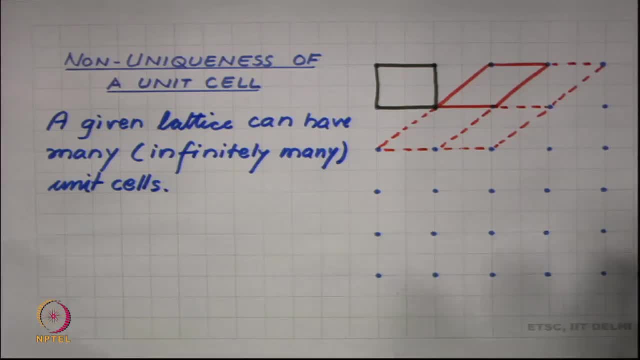 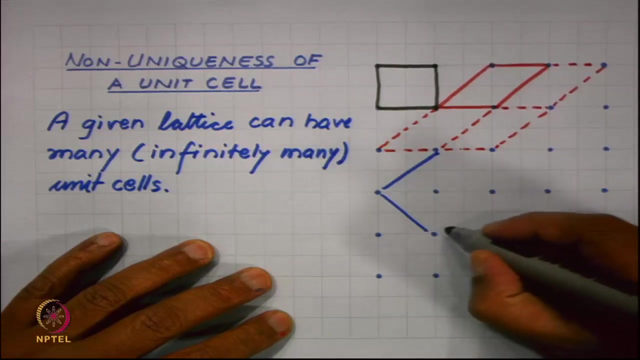 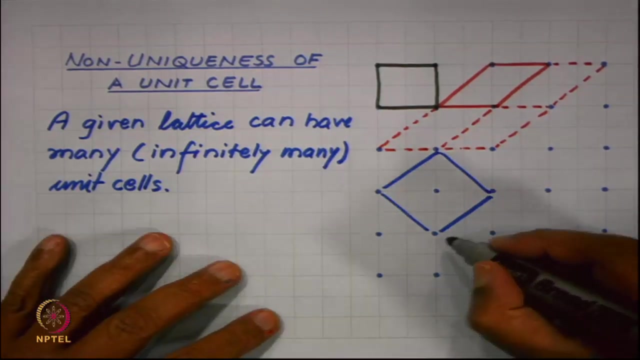 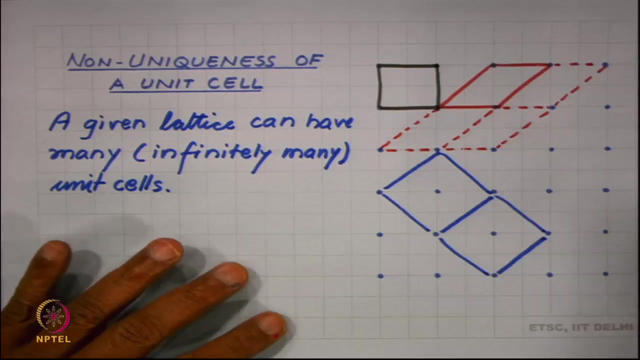 Okay, And I can change it. What happens? Also? we can select larger unit cell. for example, if I show this, I can select a larger square in which now lattice points are not only at the corners but also in the center of this. 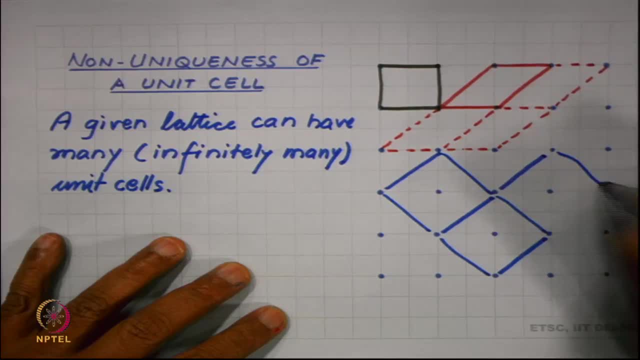 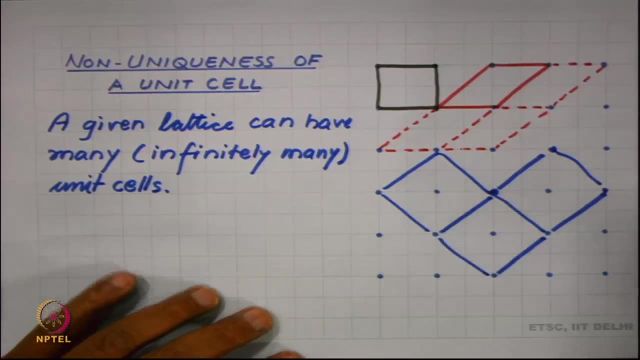 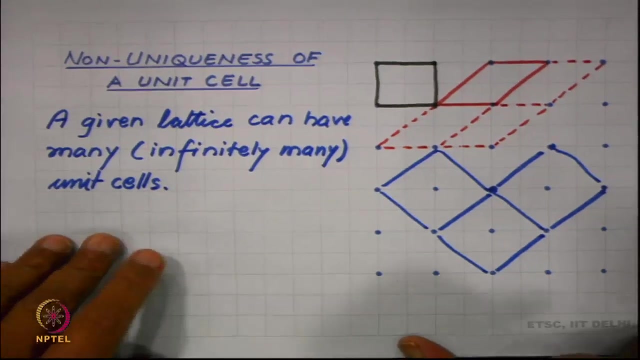 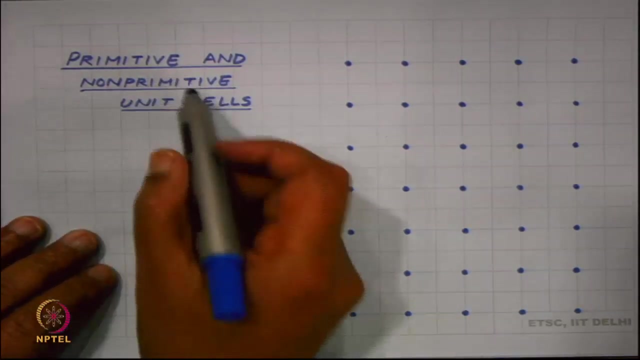 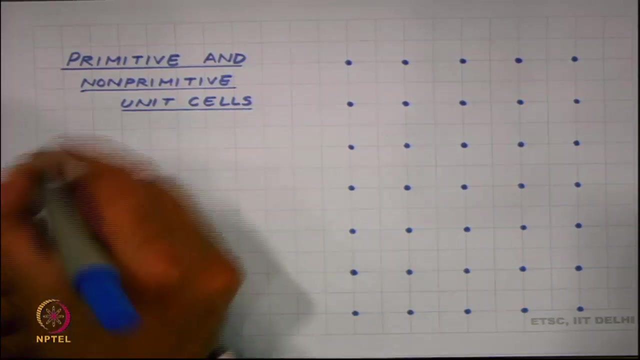 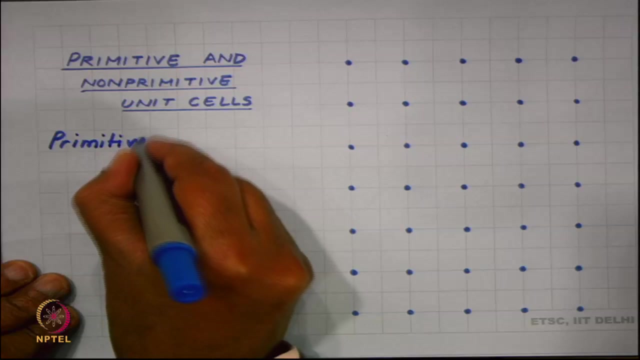 square. this is also possible. So we have many different unit cells for the same lattice. Okay, So the unit cells which I showed you can be classified as primitive and non-primitive unit cell. So any unit cell- so let us define that primitive unit cell- will have lattice points. 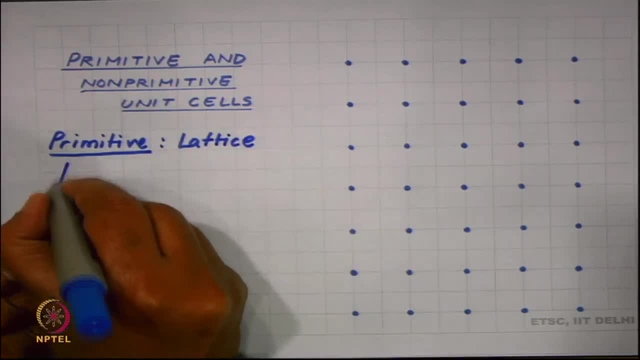 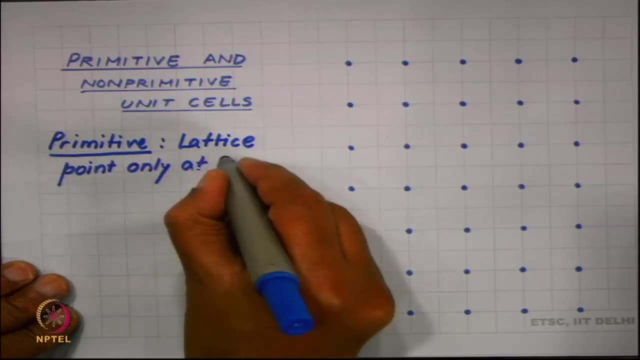 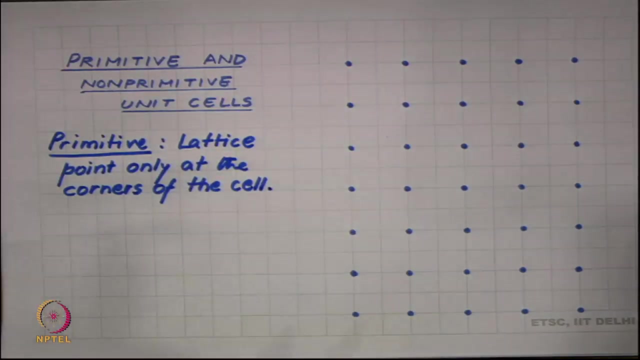 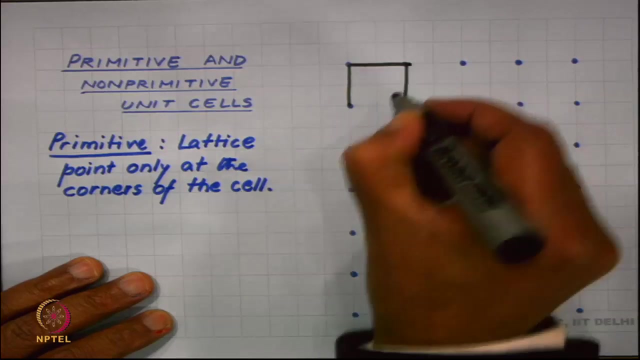 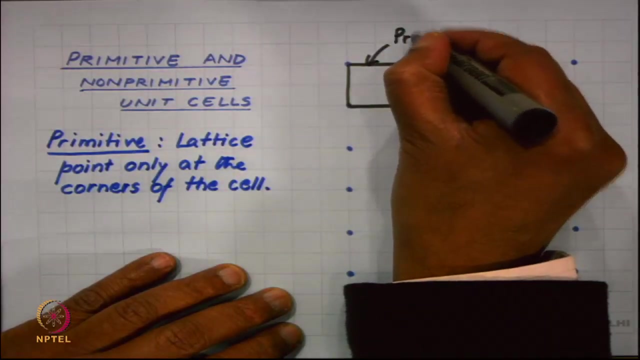 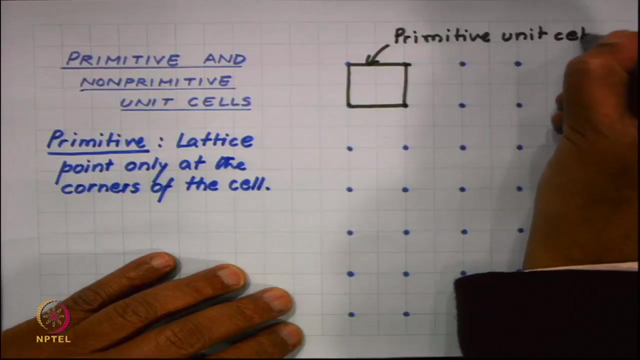 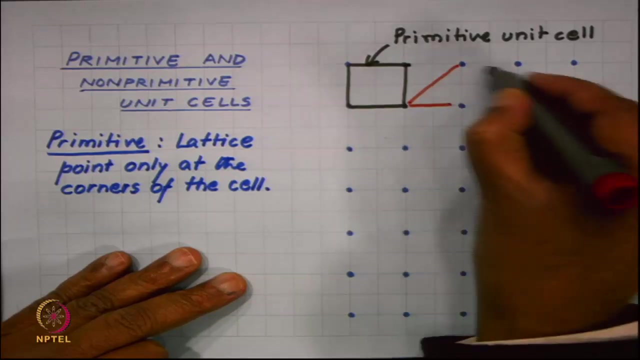 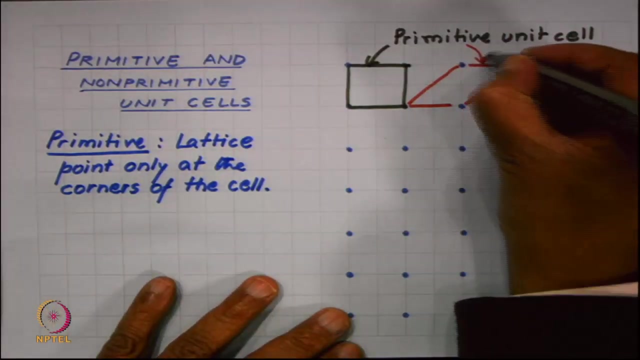 only at the corners. Okay, Only at the corners of the cell. so we have already seen, for example, the square unit cell, which we selected, will qualify as a primitive unit cell. Okay, Okay, Okay. The red unit cell, the parallelogram unit cell, this is also a primitive unit cell, because 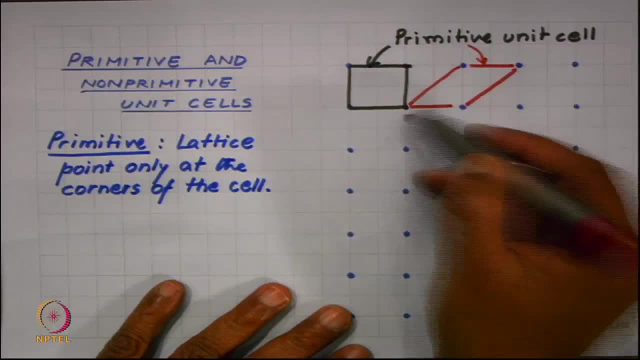 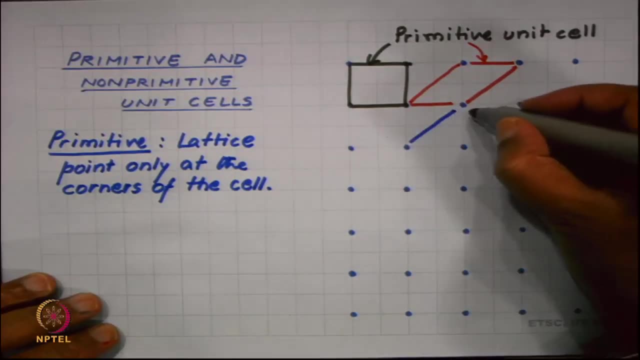 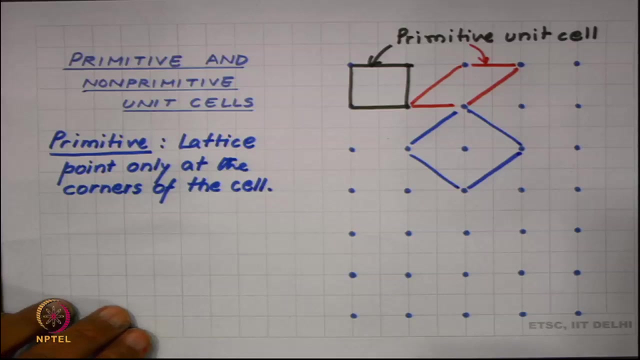 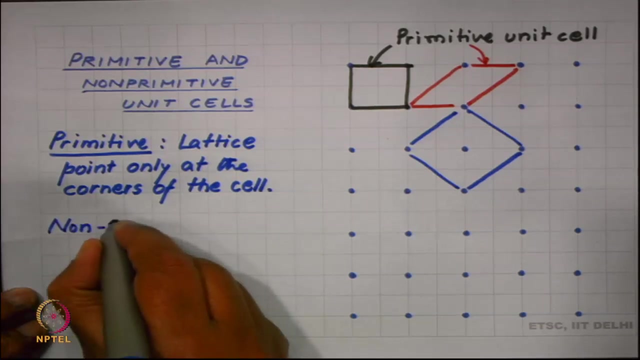 by this definition. this also has lattice points only at the corners. Okay, Okay, But the larger blue unit cell which we had selected last time, this will be an example of a unit cell which is not primitive, So the non-primitive unit cell. 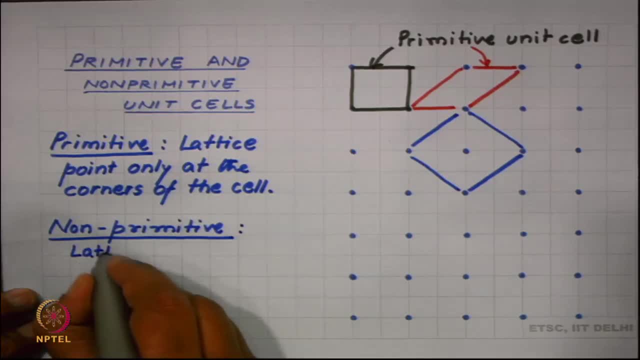 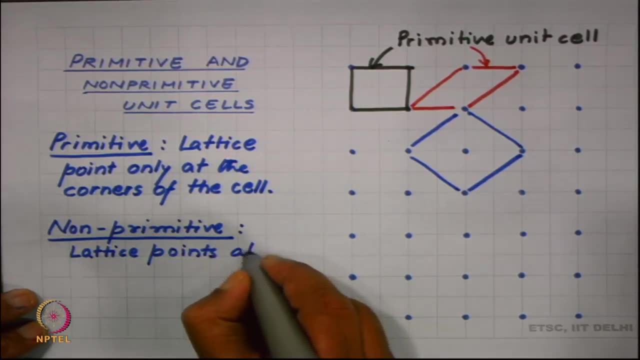 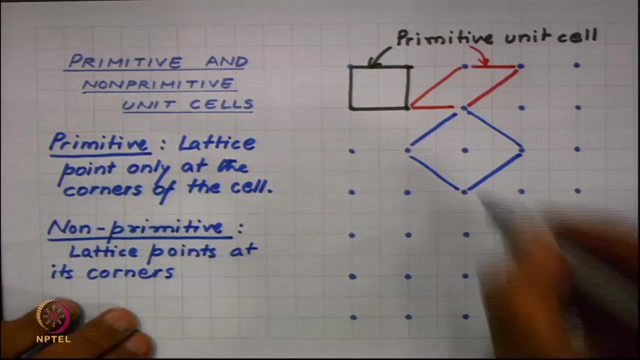 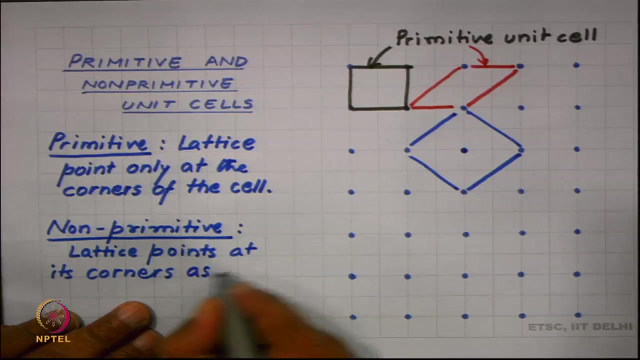 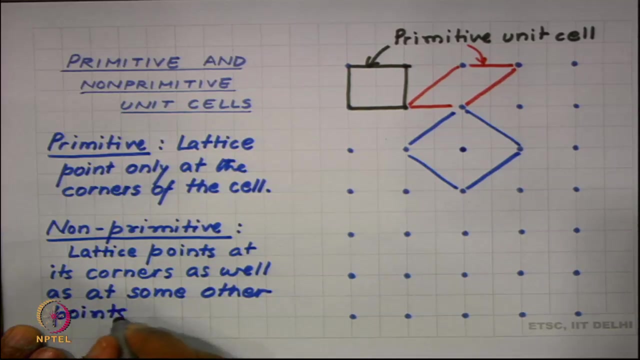 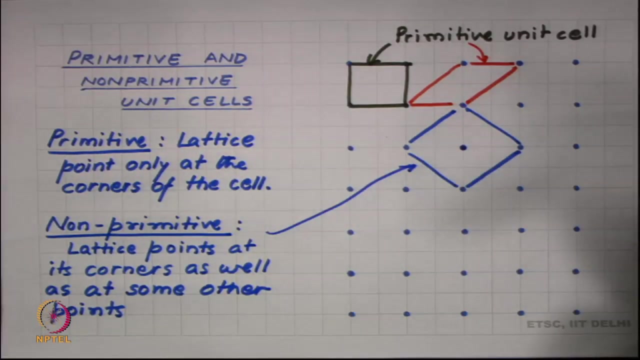 Okay, Okay, So the non-primitive unit cell- non-primitive- will also have lattice point at its corner, but it will have some lattice points other than the corner points as well as lattice points. Okay, Okay, So this will be an example of a non-primitive unit cell, and both you can have many different. 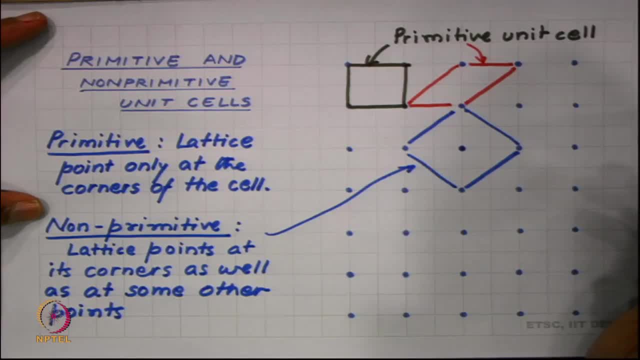 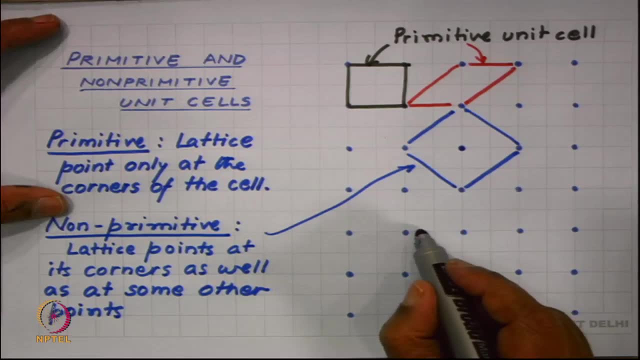 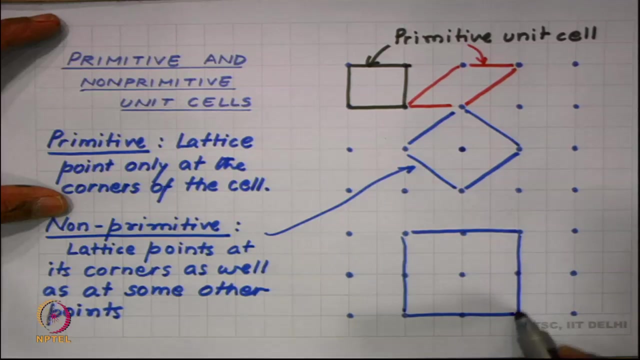 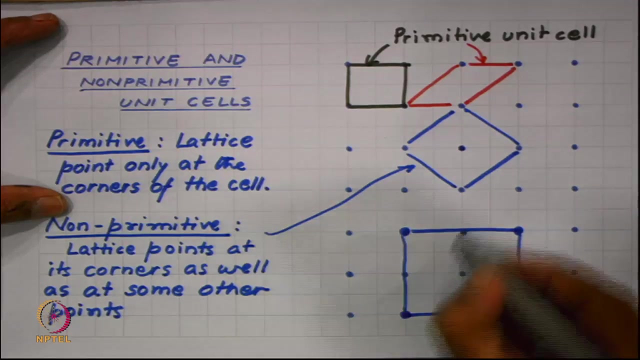 primitive unit cells. you can have many different non-primitive unit cells as well, Okay, Okay, If I choose a still larger square, let us say like this: this also is a parallelogram with lattice point at its corner, so it qualifies as a unit cell. 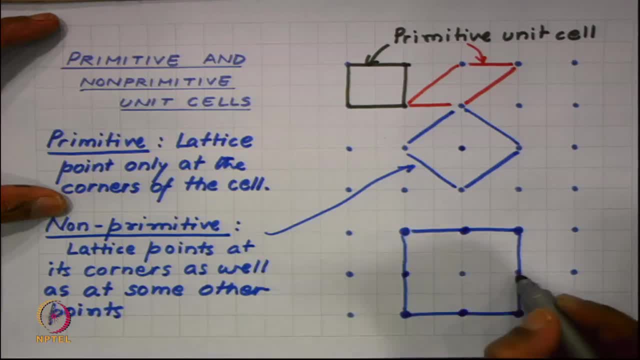 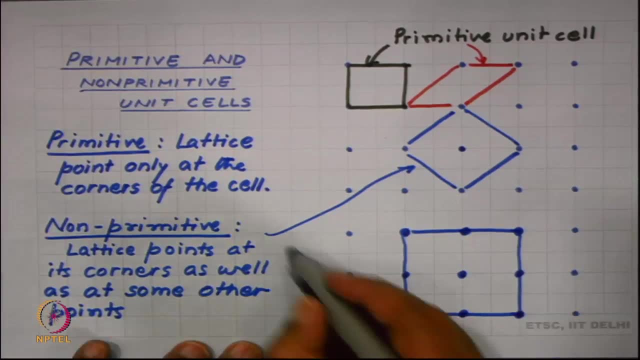 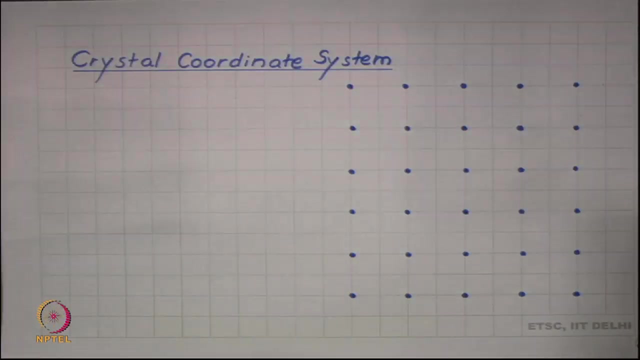 But apart from the corners, it has lattice points at its edges and it has lattice point at its center. So this will be another example. So this is another example of non-primitive unit cell. We now define what is called a crystal coordinate system. 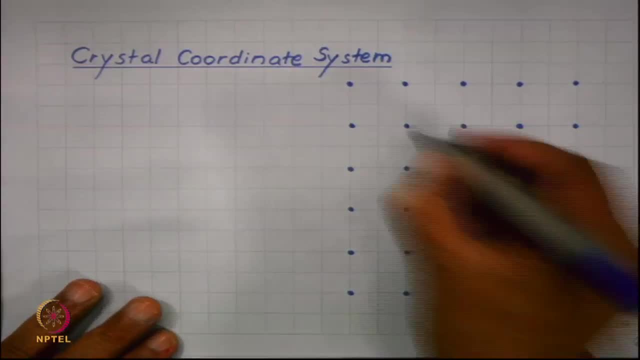 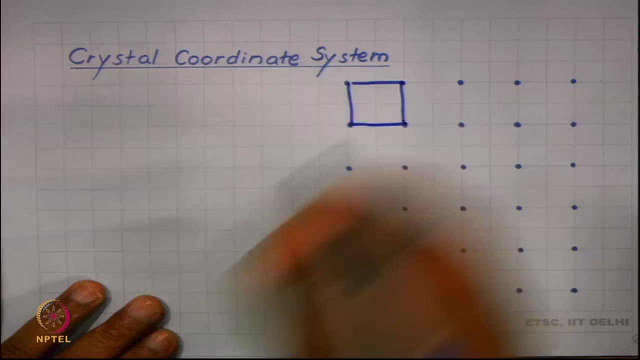 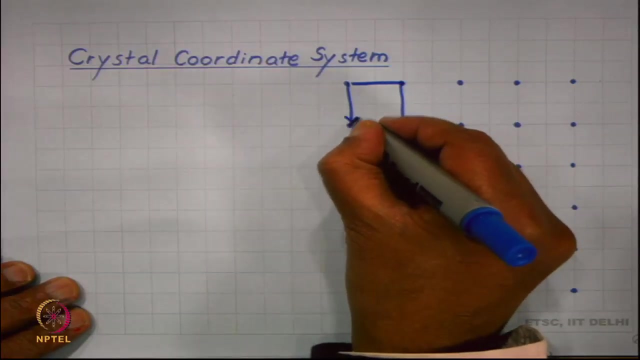 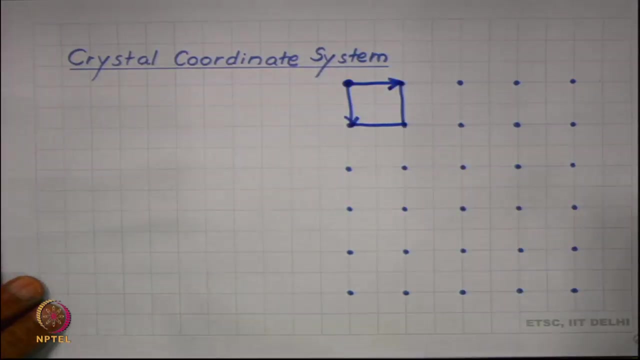 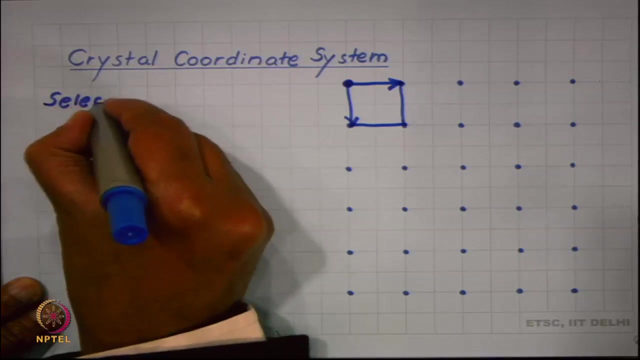 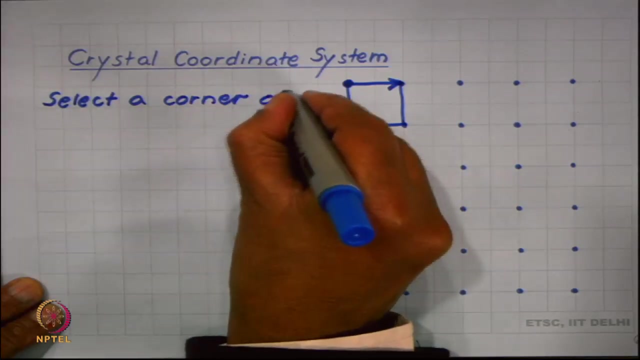 Once we have selected our unit cell, let us select the unit cell. so unit cell itself, parallelogram or parallel pipette unit cell? Okay, So the unit cells are defined by the vectors along its edges. So select a corner of the unit cell. 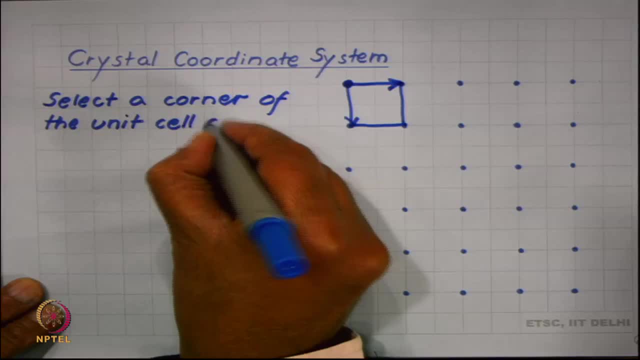 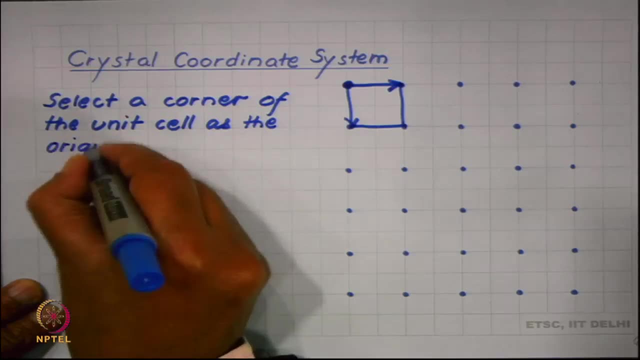 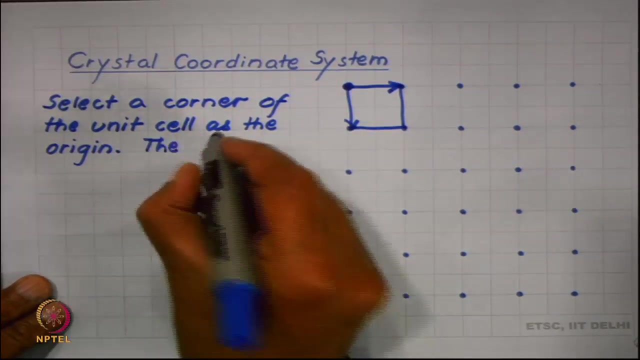 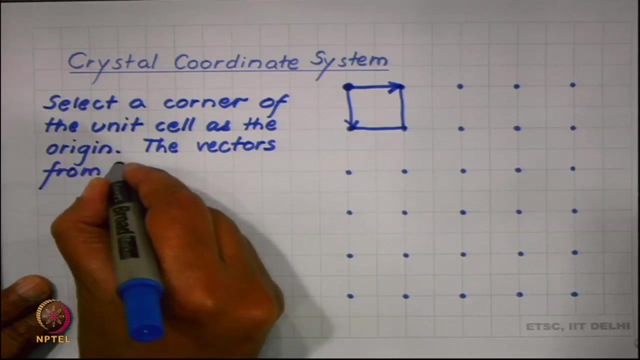 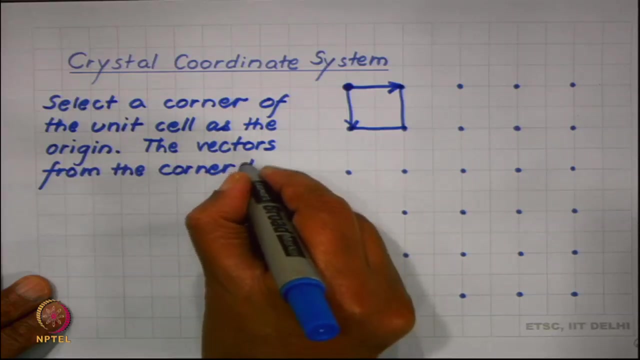 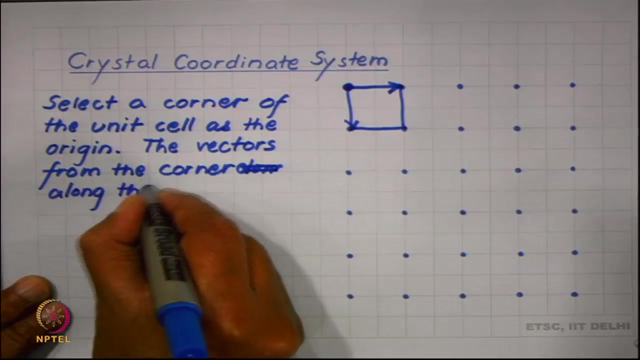 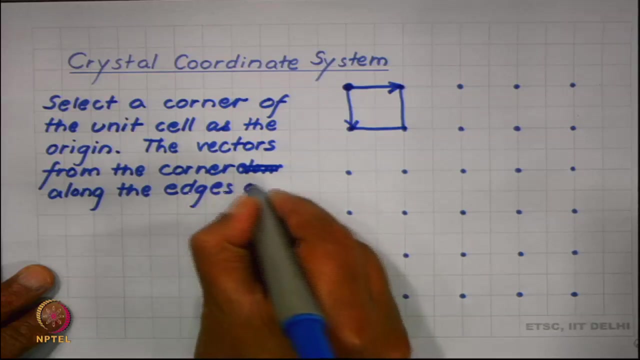 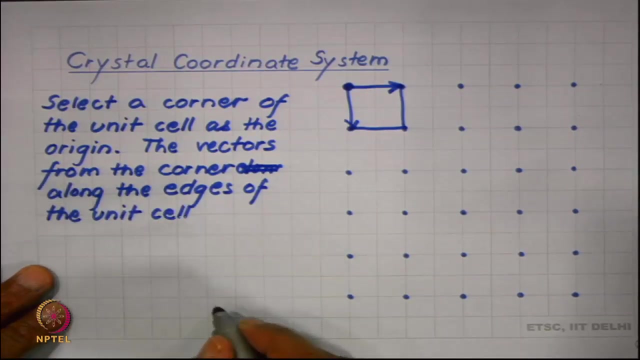 Okay, Okay, Okay. So the unit cell is defined as the origin. as the origin, The vectors from the corner of the unit cell are defined by the vectors along its edges. Okay, Okay, Okay. So the unit cell along the edges of the unit cell is defined as the non-primitive unit. 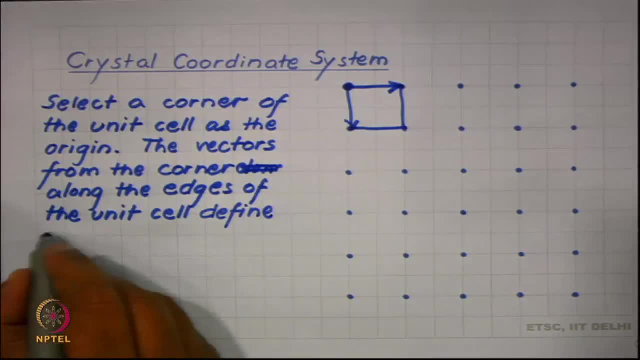 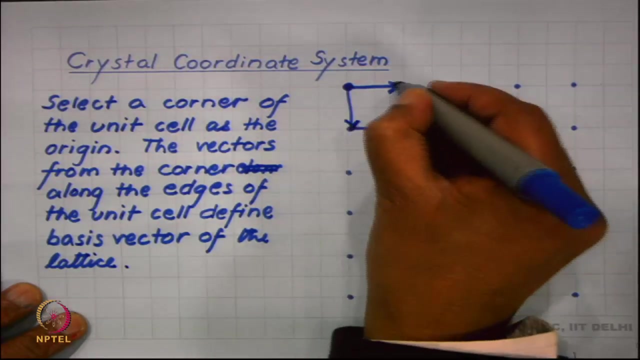 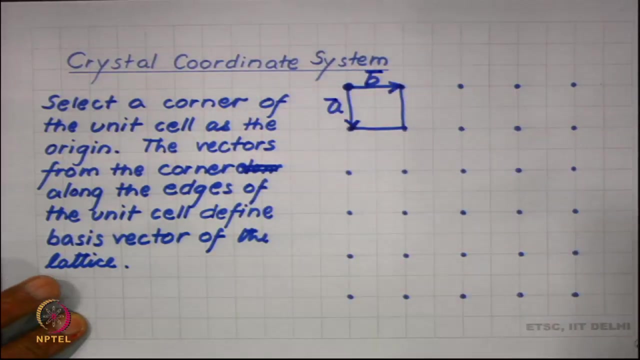 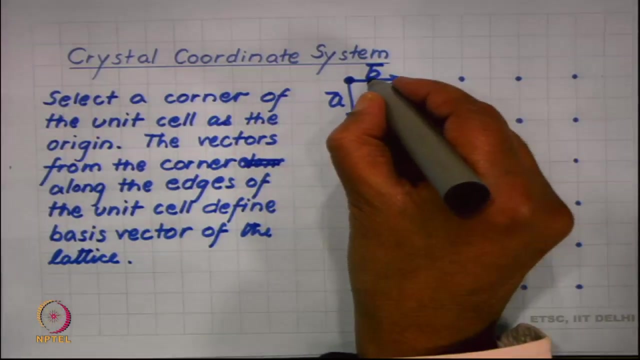 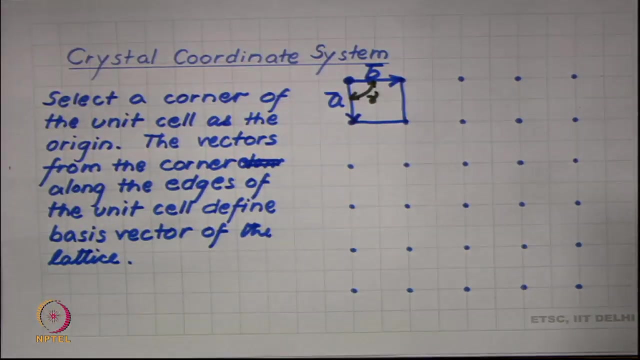 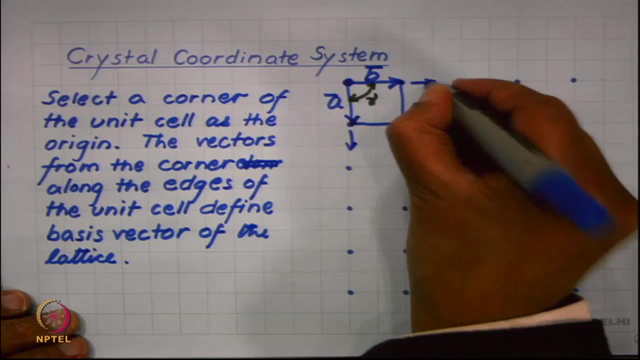 cell. Okay, Okay, Okay. So we have selected this as the origin. along the edges we have these two vectors, a and b. So a and b becomes the angle between them is gamma. We can select, We can select, So we can also define these as the axes. this is our x axis, this is our y axis, this 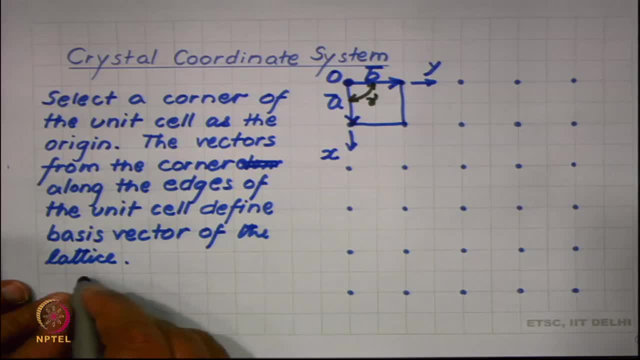 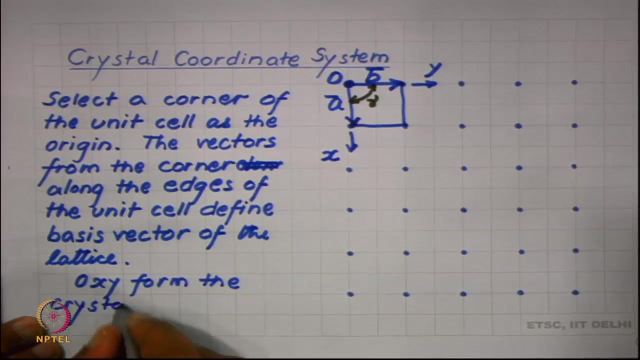 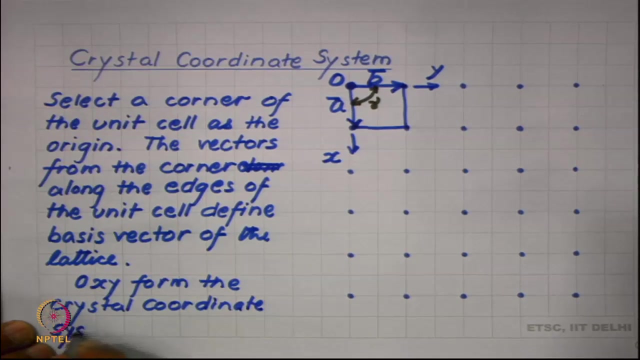 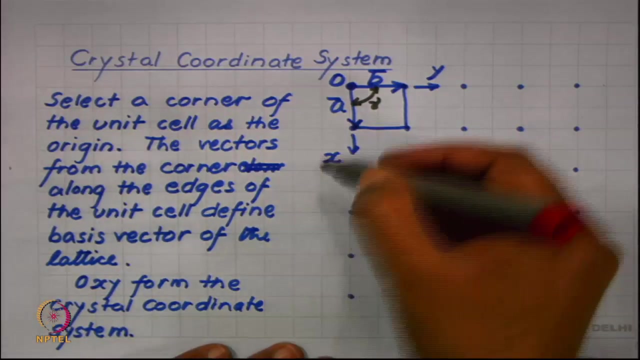 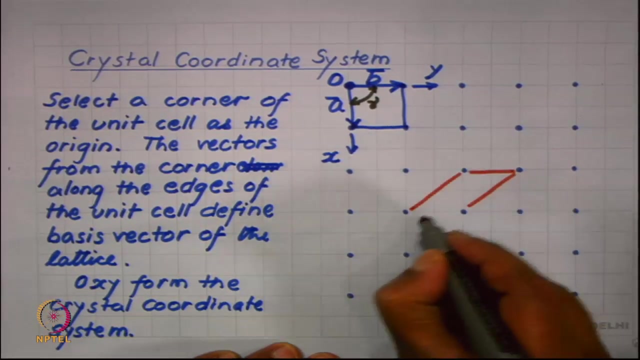 was the origin, o, So o, x, y form the. Okay, This is the crystal coordinate system. So of course the crystal coordinate system is associated with the selection of a unit cell. So if we select a different unit cell, for example if we select this parallelogram unit, 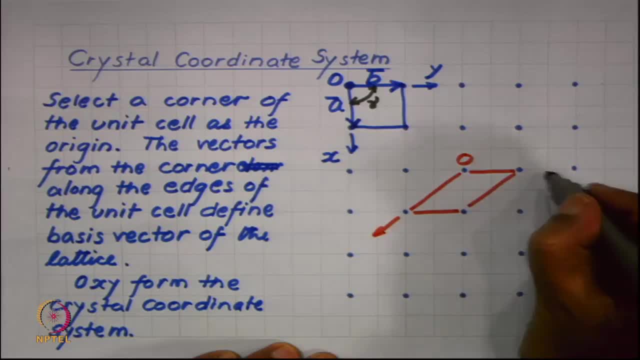 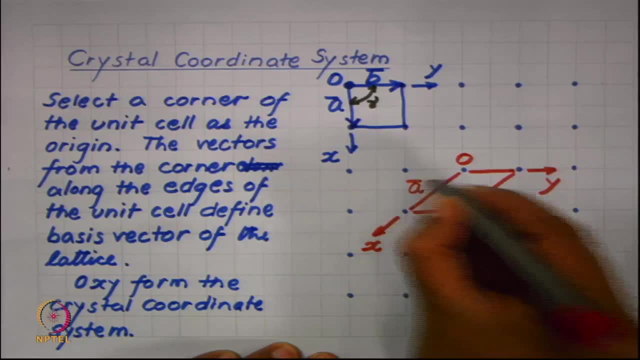 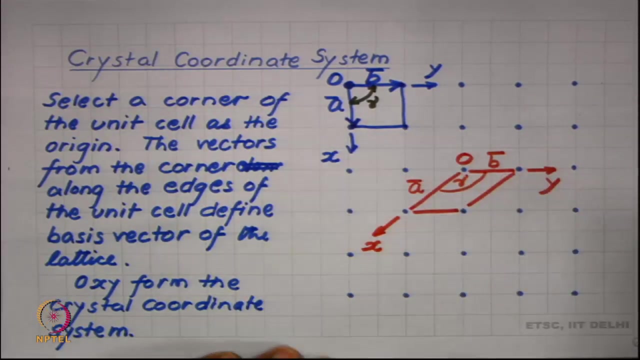 cell, then my x and y are no more orthogonal. my a and b are also not equal, Okay, Okay, Okay, So b is exclusive to b. Yes, Because b is own, equal to the z and the angle gamma. it is not 90 degree. 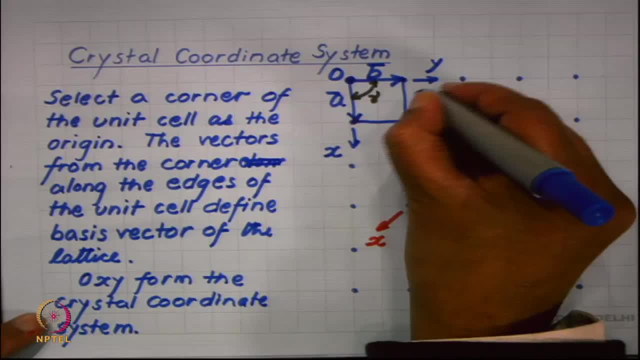 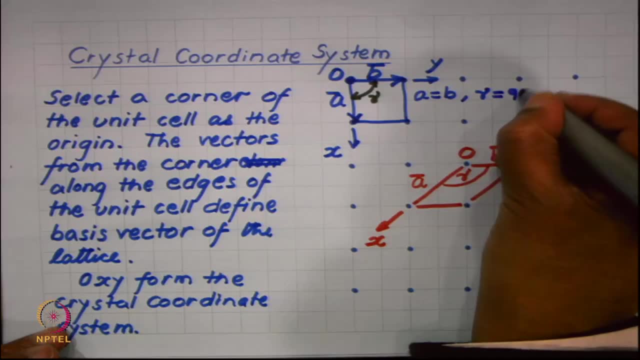 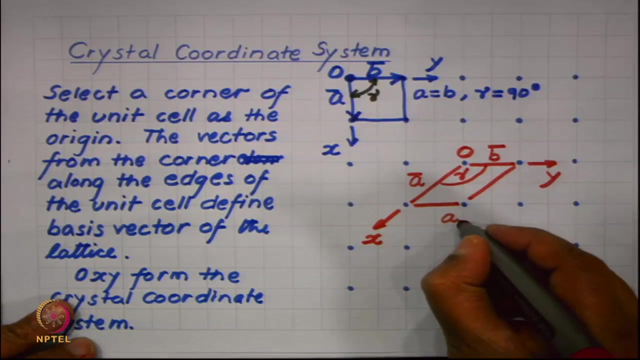 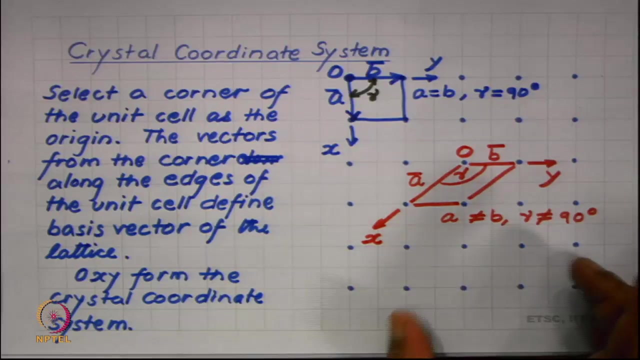 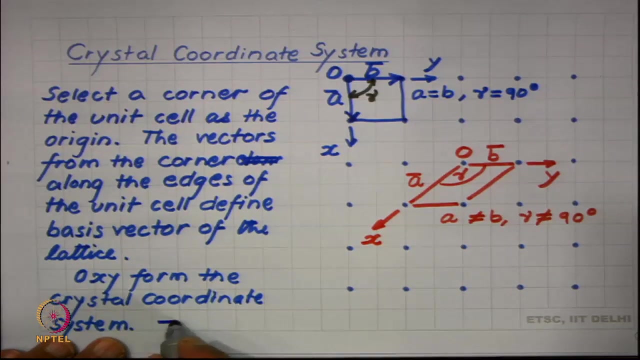 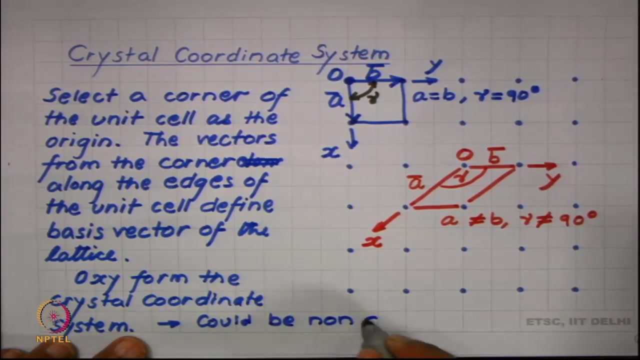 So in this case a was equal to b and gamma was 90 degree. but here for the same lattice, I have now selected a different coordinate system where a is not equal to b, Okay, And gamma is not equal to 90 degree. so crystal coordinate system can be non Cartesian could. 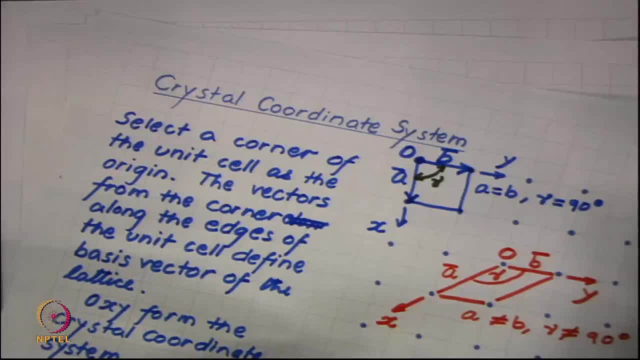 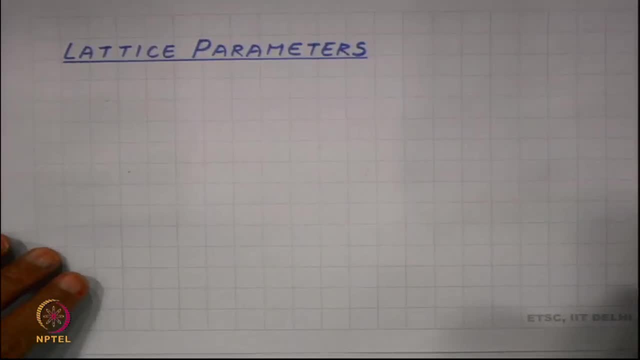 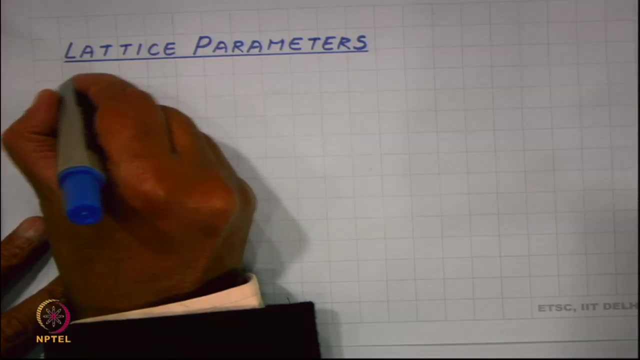 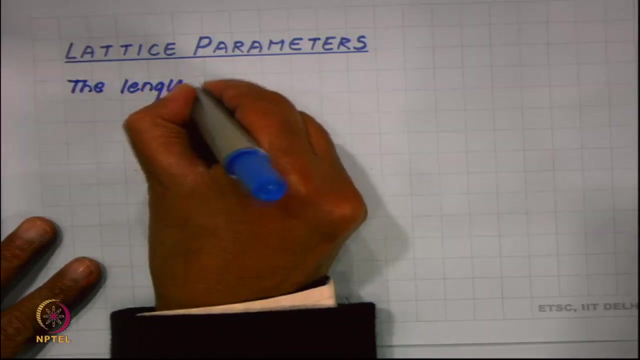 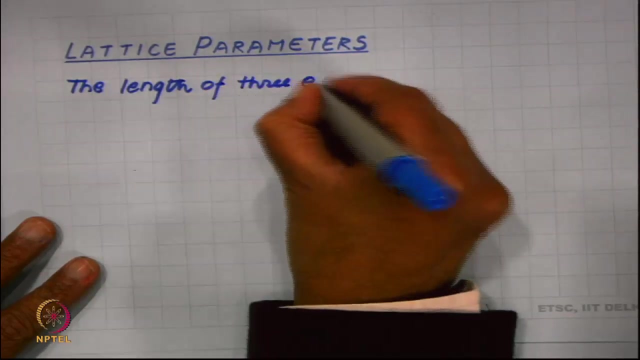 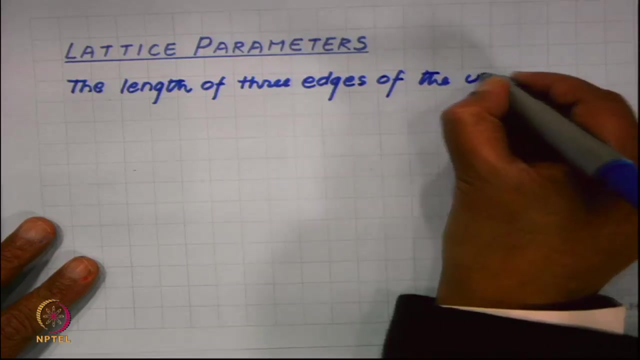 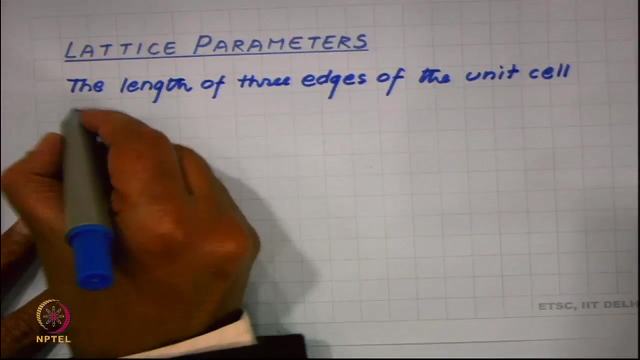 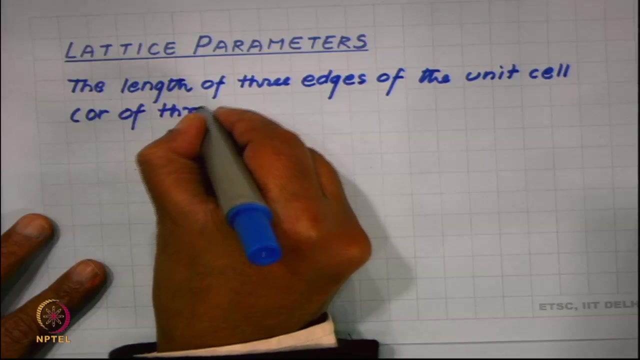 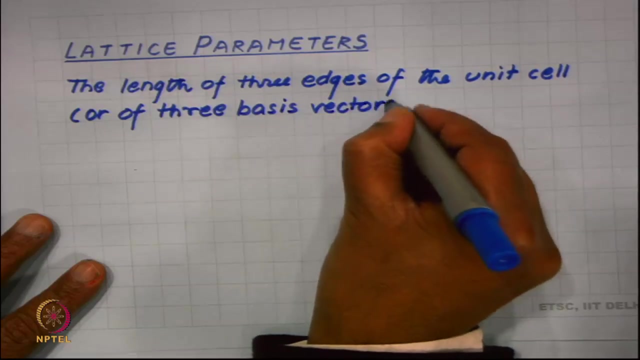 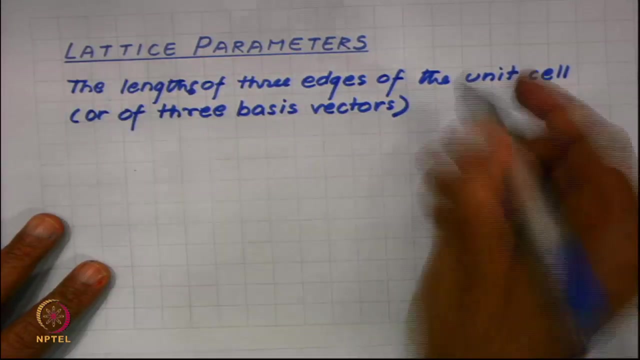 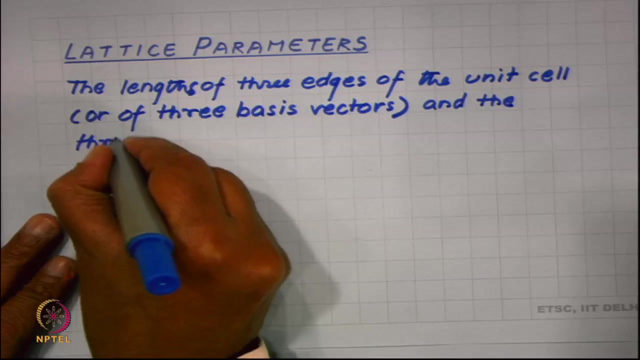 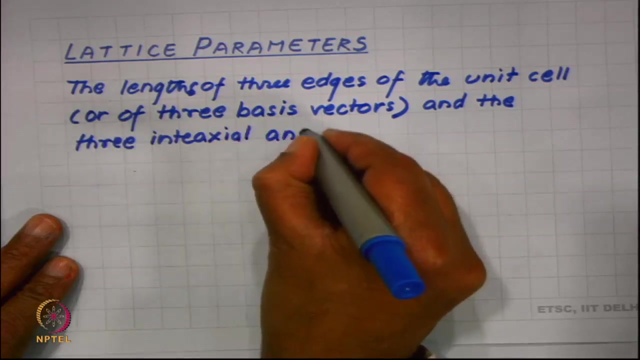 be non Cartesian. We now will define the lattice parameters. so, for any given unit cell, the length, the length of 3 is of the unit cell, or in other words, of the 3 basis vectors, The length, the lengths of 3 edges of the unit cell or the 3 basis vector, and the 3. 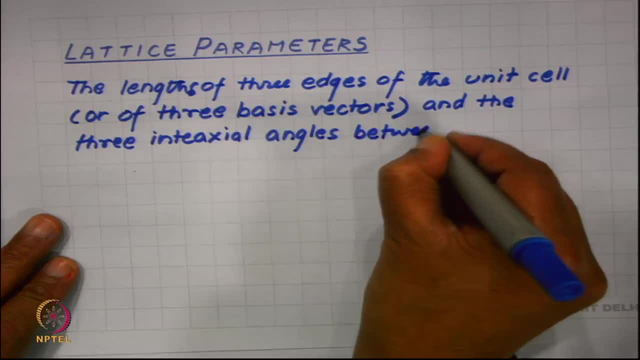 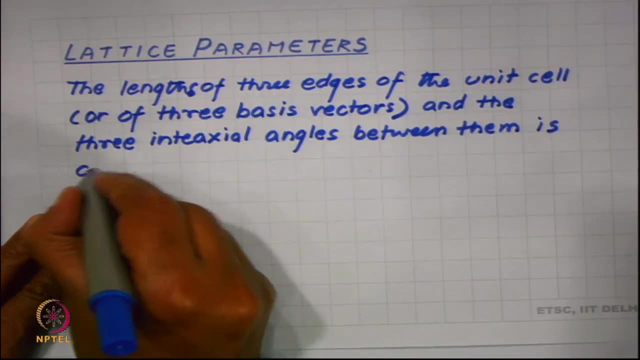 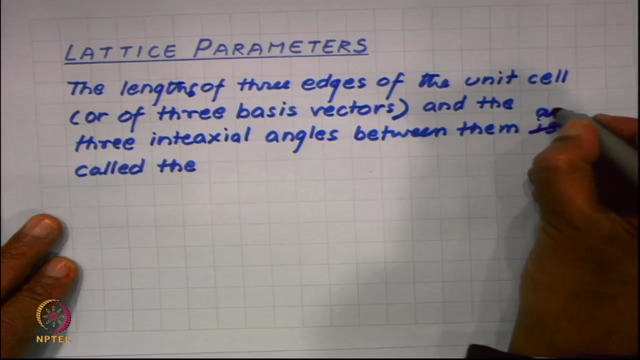 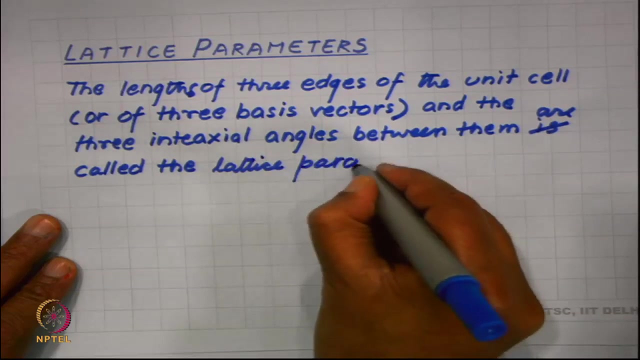 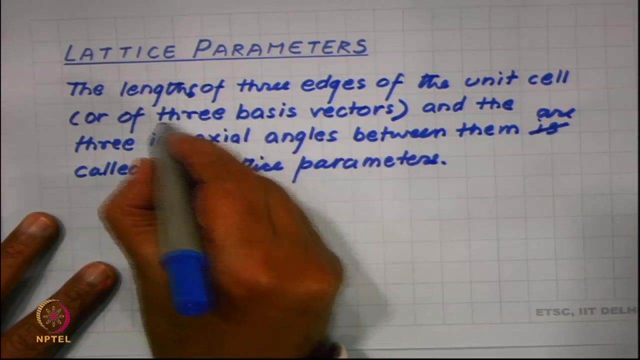 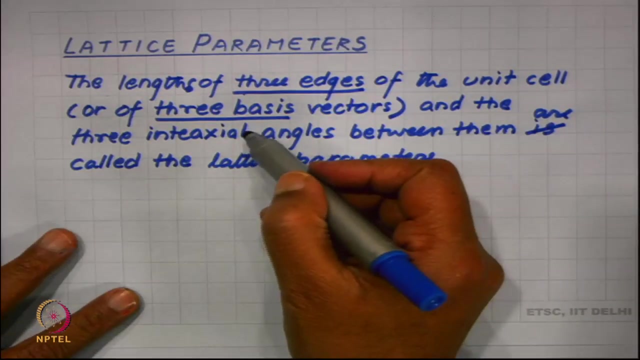 inter axial angles between them, Well, are called the lattice parameters. Now I am talking in 3D, so that is why we are talking of 3 basis vectors, 3 edges and so on. Of course, in 2D there will be 2 basis vectors. 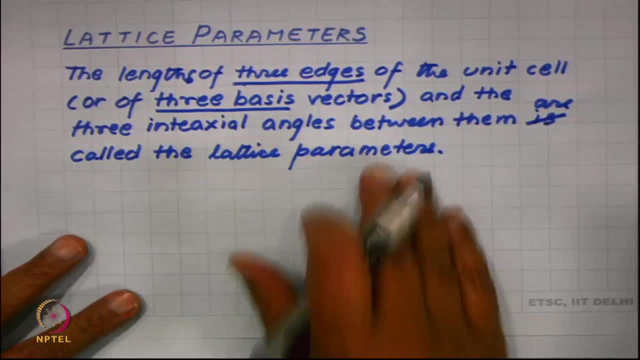 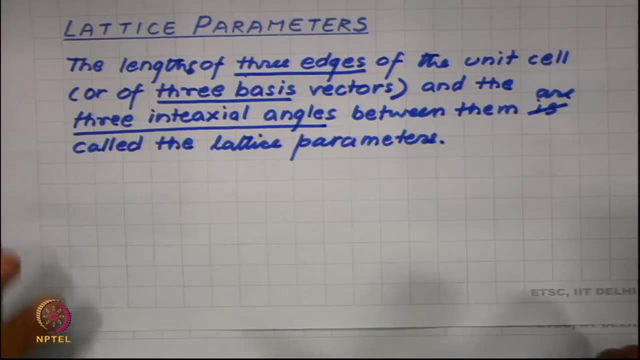 So there will be 2 basis vectors and 2 edges and there will only be 1 angle, 3 triaxial angle in 3D, 1 angle in 2D. So let me try to draw a parallel piped unit cell to define these. 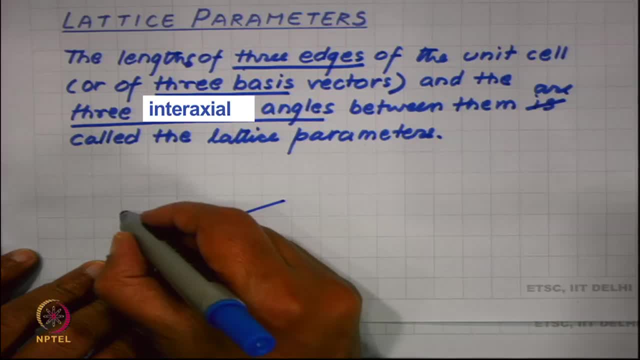 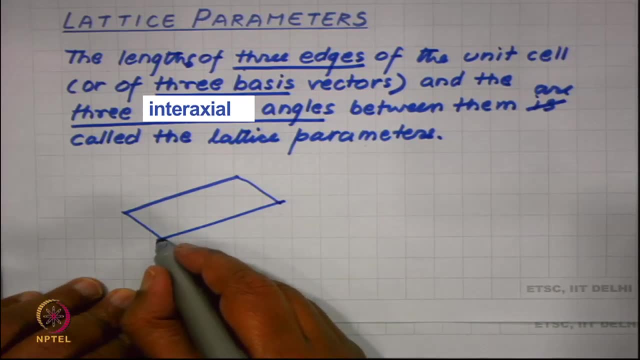 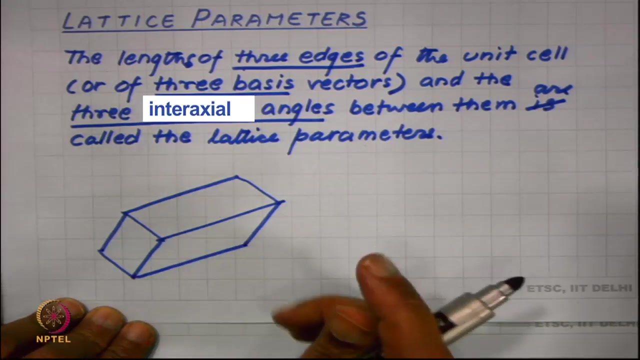 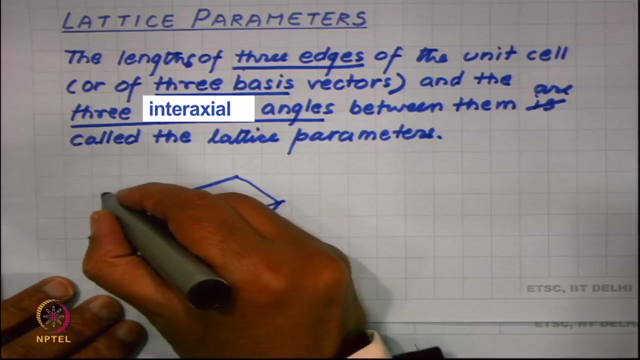 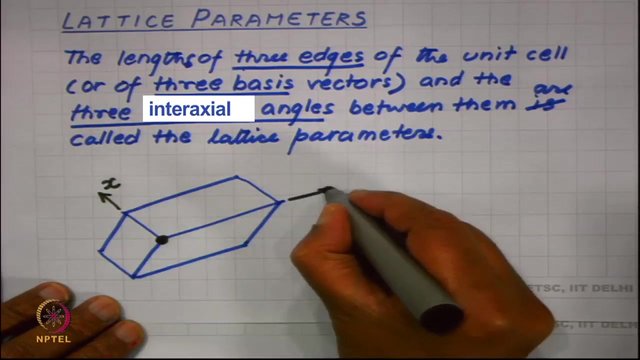 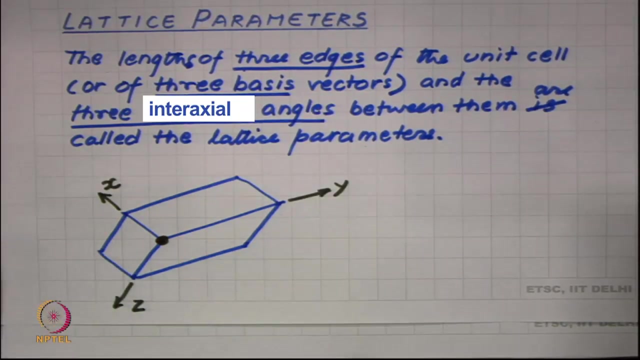 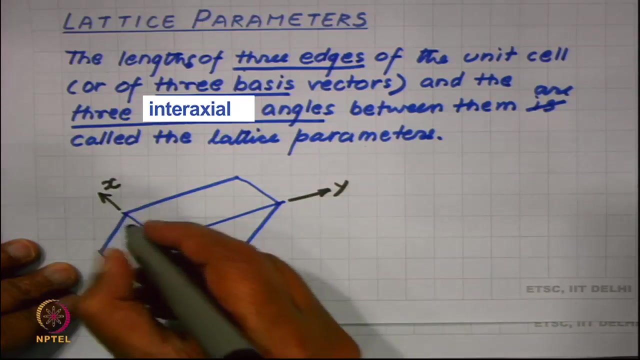 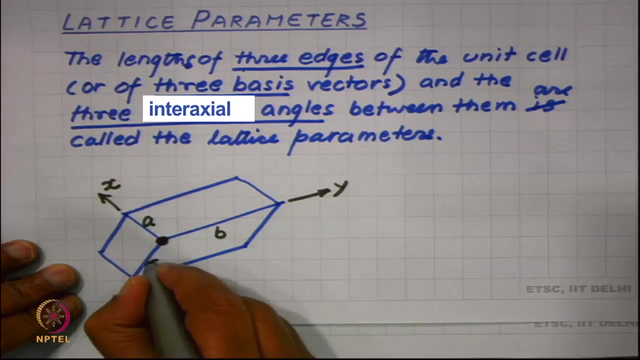 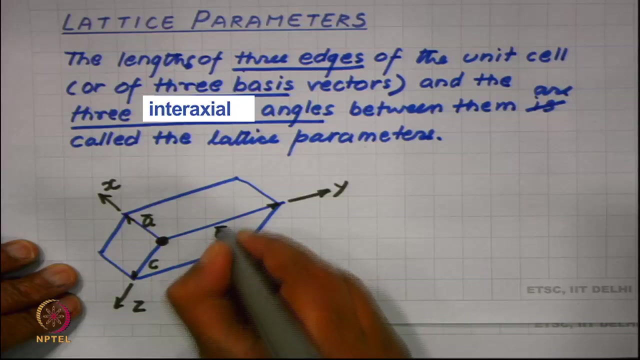 So suppose I have a parallel piped unit cell And I choose this as my origin and choose this as my x-axis, y-axis and z-axis. so they are not necessarily orthogonal and the corresponding length a, b and c. these are also not necessarily 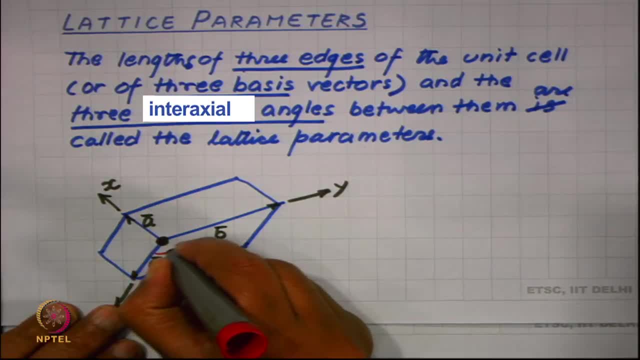 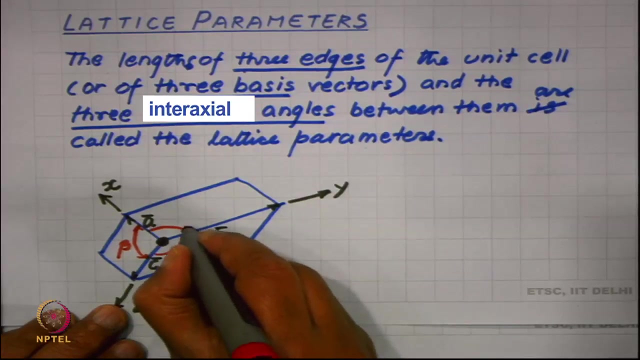 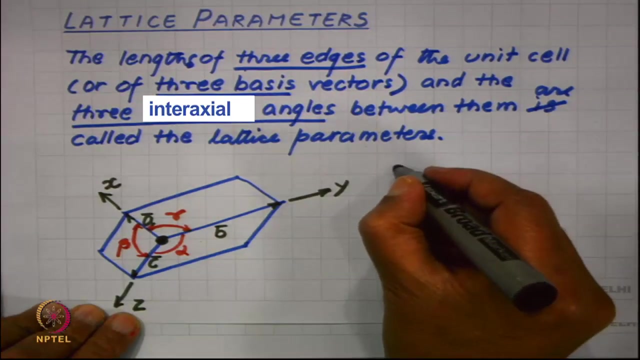 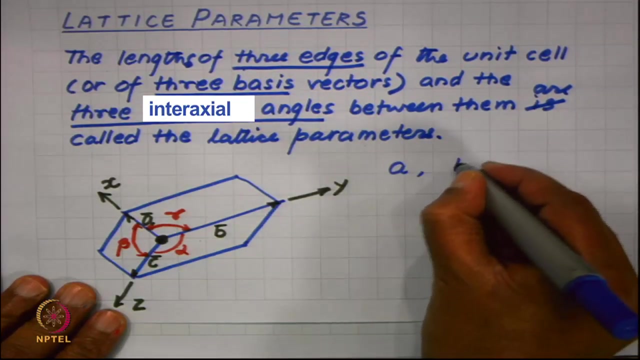 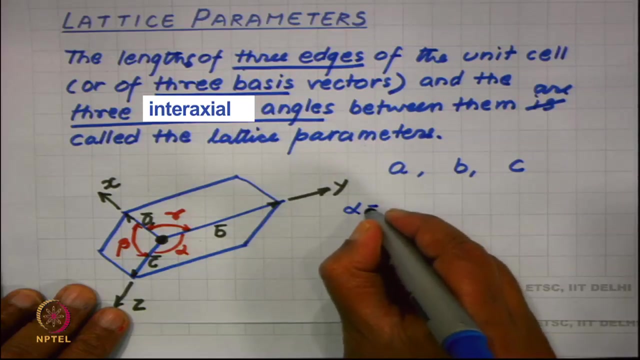 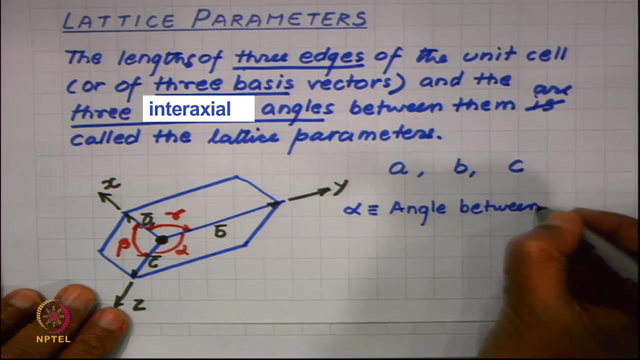 equal and we have three angles: Angle between b and c, alpha, Angle between a and c, beta and angle between a and b- gamma. so the three lengths a, b and c And the three angles are like this: Alpha angle between b and c, beta angle between c and a, gamma angle between a and 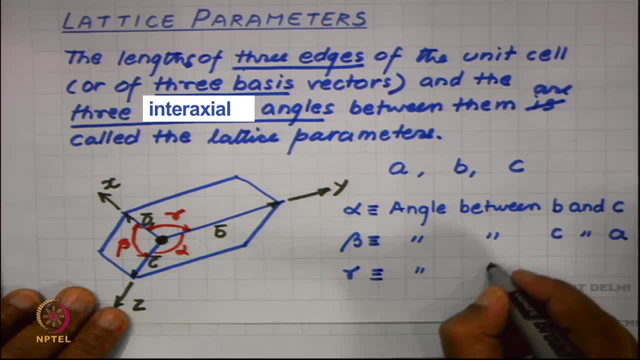 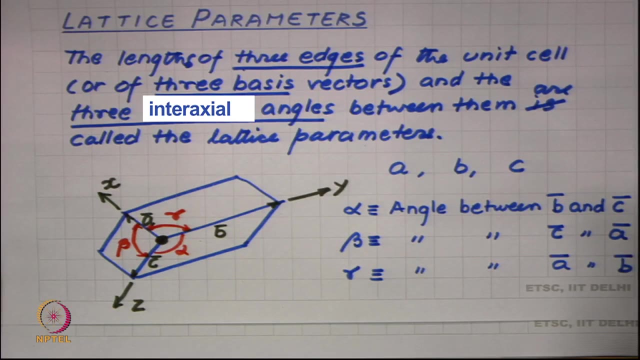 b, Okay, Okay, This is the convention of naming. alpha is always taken to be angle between b and c, and so on. So once these six numbers are given, we have the complete description of the so called lattice parameters of the crystal. 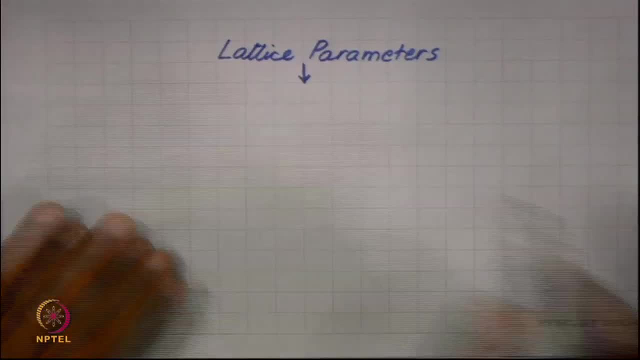 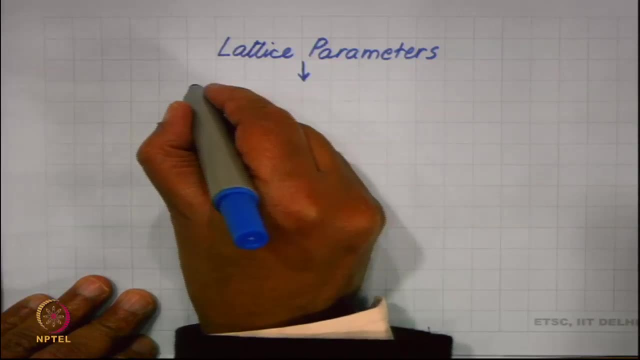 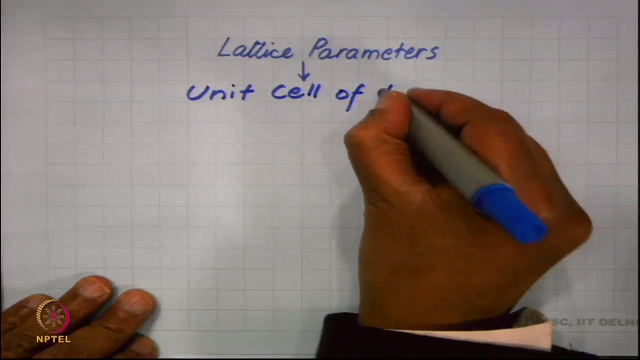 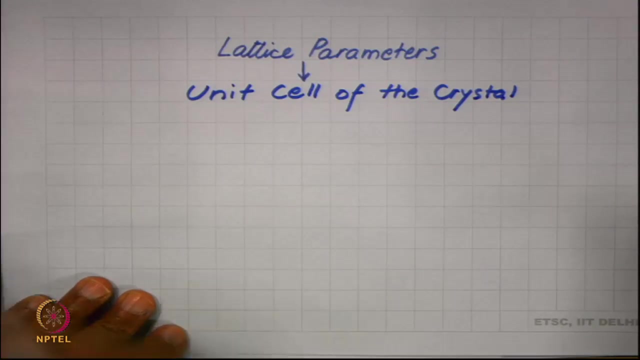 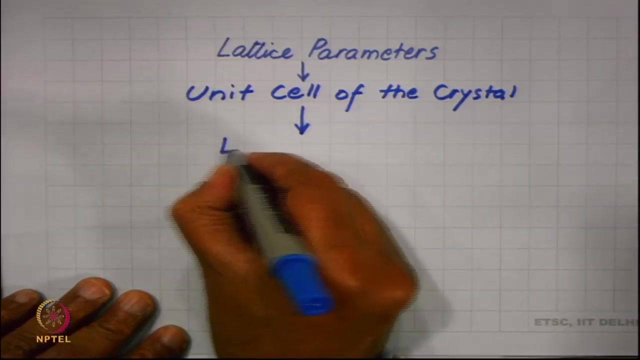 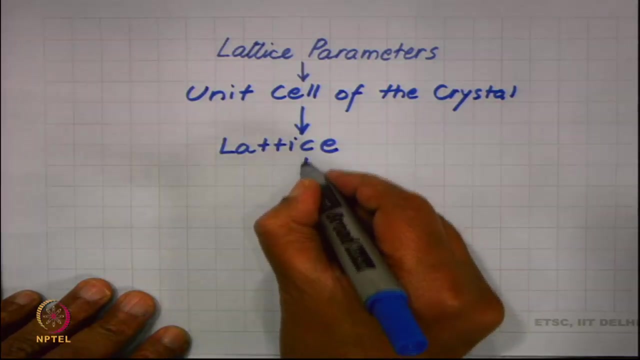 Okay, Which means if we are given the lattice parameters, then we can construct the unit cell of the crystal. If we know the unit cell by repetition of the unit cell, Then we know the lattice, and if we know the lattice, then we have the information. 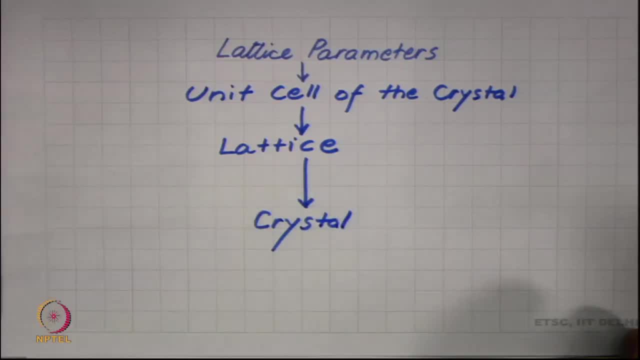 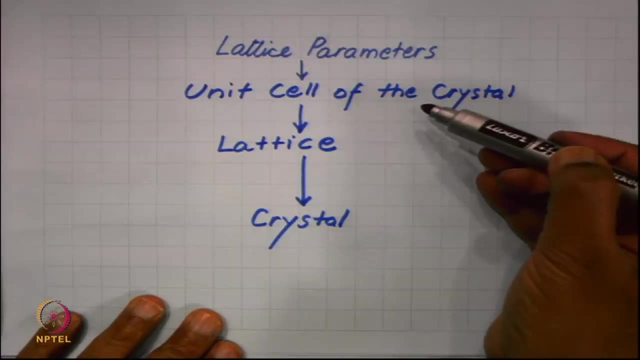 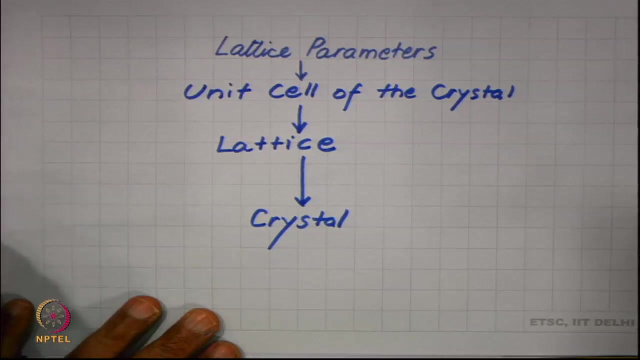 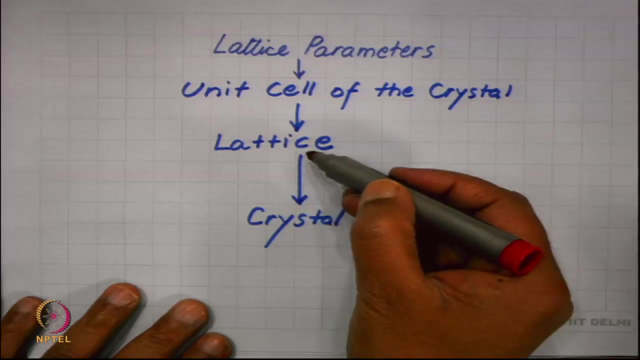 about crystal or am I making a mistake here? Lattice parameter gives me the unit cell, unit cell gives me the lattice, but lattice gives. So if you have been following this video till now, you will be worrying about this lattice from lattice going to crystal, because we have said lattice only gives me what. how? 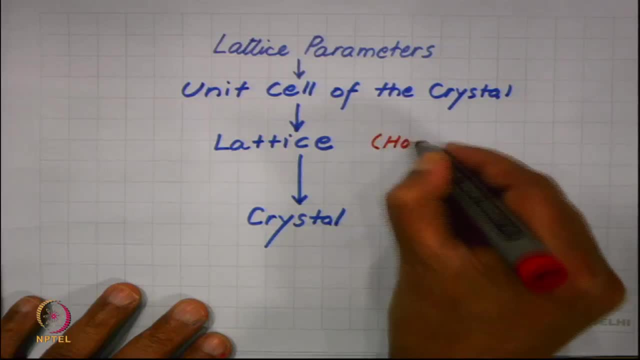 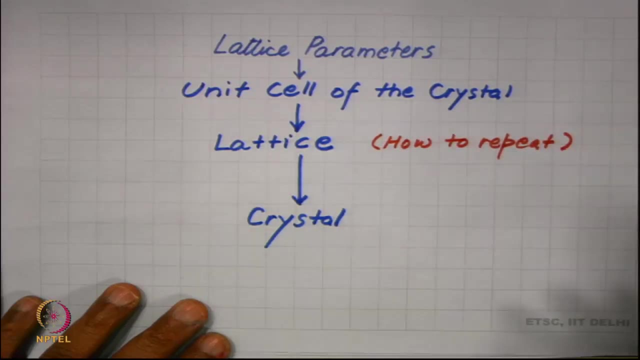 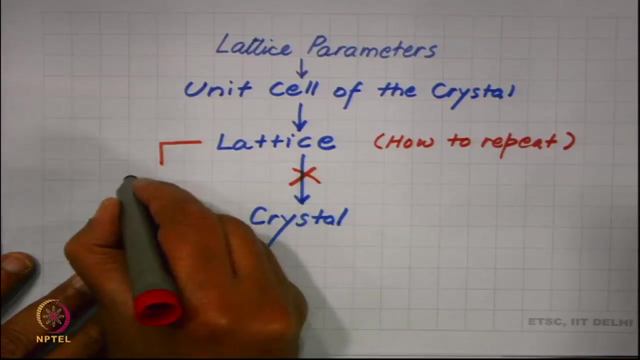 to repeat. lattice gives me, but it is not giving me what to repeat, and unless and until I know what is being repeated, that is, unless and until I know the motif. I do not know the crystal. So this is not right. I have to come through. I need the information about motif. so if 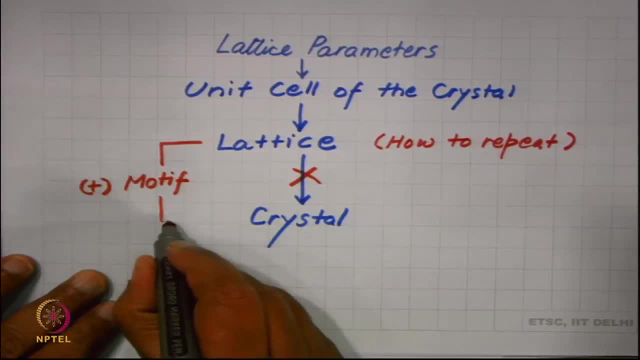 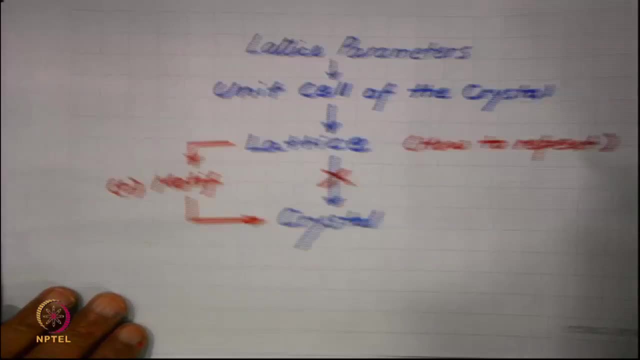 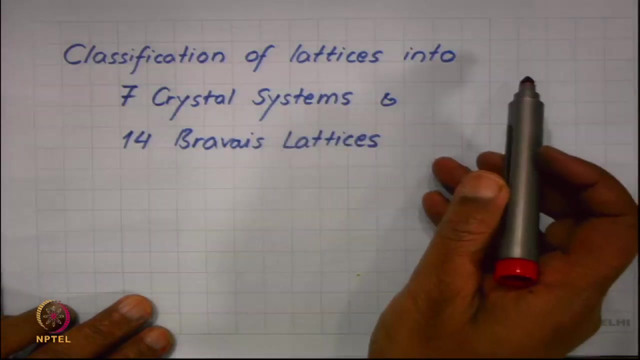 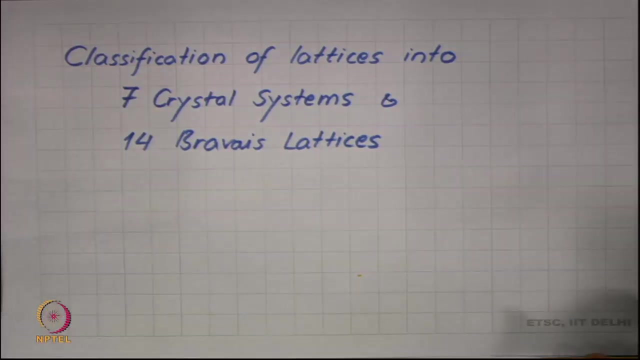 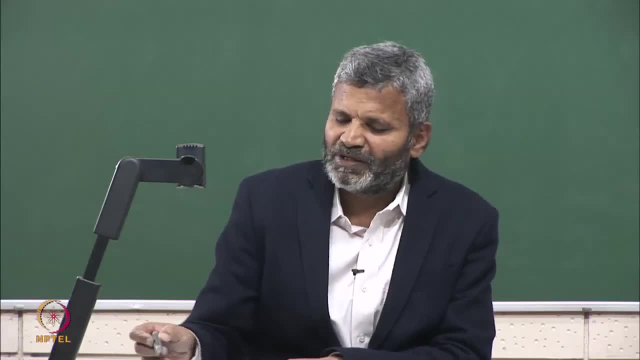 Thank you, So thank you. The next topic will be classification of lattices into 7 crystal systems and 14 Brevet lattices.